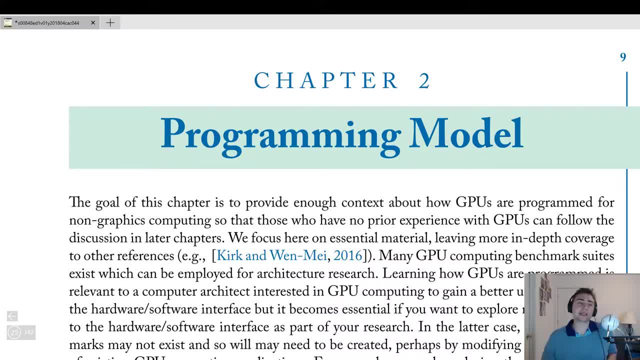 where GPU programming came from for general-purpose applications, followed by you know what does a GPU look like from kind of a 10,000 foot view, as well as some basics like the history, and you know what kinds of GPUs are out there, whether they're discrete or whether they're integrated, so you know they're. 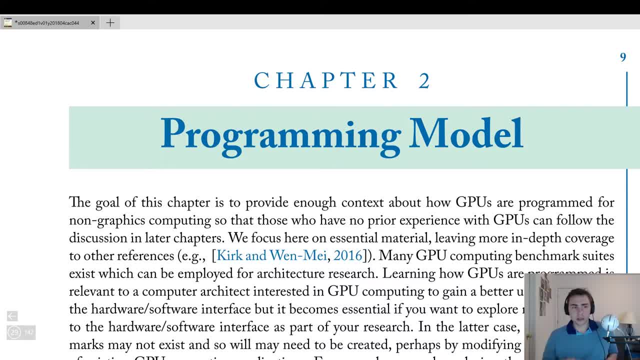 connected with the same physical memory with as the CPU. So you know, in order to understand the architecture that we'll cover in later videos, we have to understand the programming model for GPUs. This is really essential before we dig into the hardware because, at the end of the day, how we program a GPU depends. 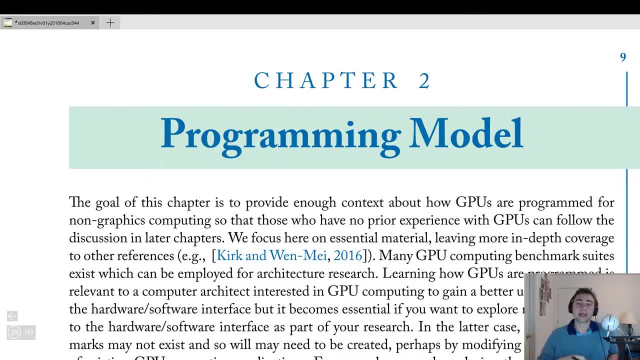 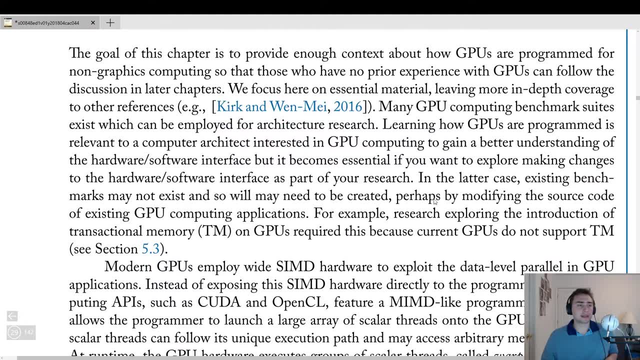 on the architecture of the GPU. So we have to understand the architecture of the GPU. We'll depend on the underlying hardware, and the underlying hardware is of course influenced by how we're able to program it. So this is just going to cover kind of the basics of GPU programming. If you're interested in, you know, GPU. 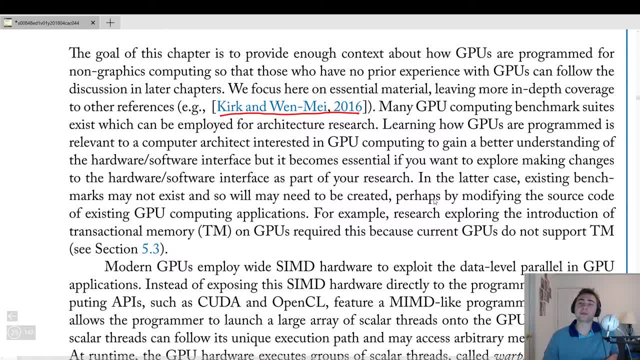 programming itself. I suggest this book which is cited here, which is Programming Massively Parallel Processors. It's a great book. I used it when I was learning GPU programming. Also, check out the videos that I have on the other YouTube series- CUDA Crash Course, where you know I do a lot of the 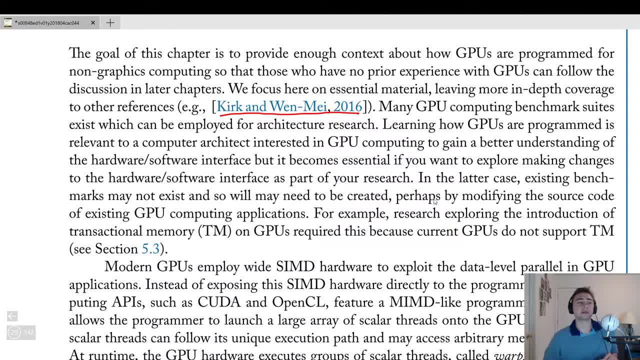 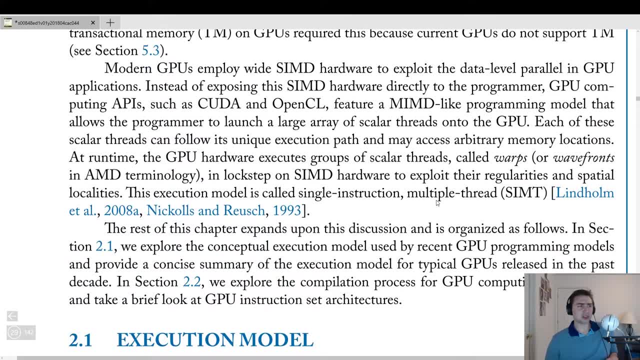 examples that they cover in this book as well, and some other things that aren't covered in the book. So you know, let's just jump right in and so and start discussing how we program GPUs. So GPUs employ wide SIMD hardware. So again, this is single instruction, multiple data to exploit data level parallelism inside of. 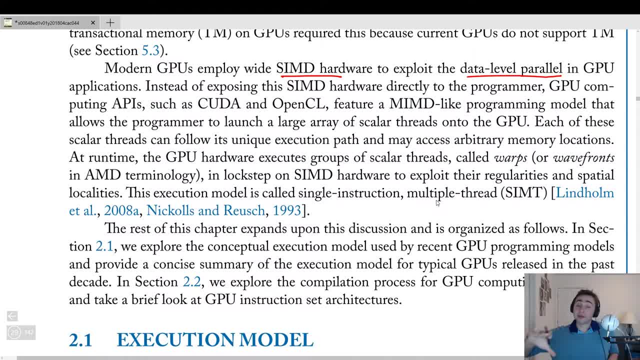 GPU applications. So you can see, here I've got a bunch of GPUs, I've got a bunch of CPUs here. So pardon the noise. We have a lot of parallelism in our data that we want to exploit, so you know we can work on different pieces of data at the same. 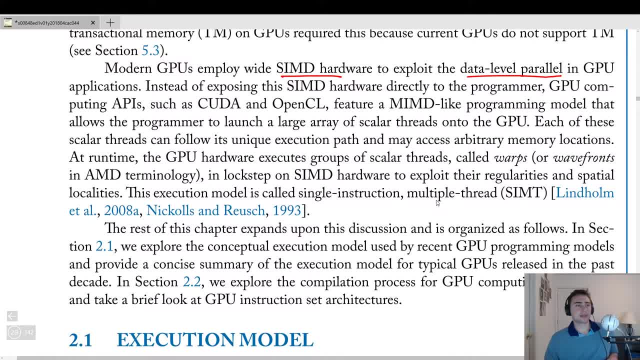 time because there's no dependencies. That's really what we use GPUs for. But how we actually program this hardware through APIs like CUDA and OpenCL. So CUDA is is from Nvidia, So Nvidia GPUs- GPUs- are typically programmed using CUDA, And then AMD GPUs- our program, you know, a lot of times with OpenCL to program it. So it's just a little bit helpful to know that there's a fair amount of parallelism. 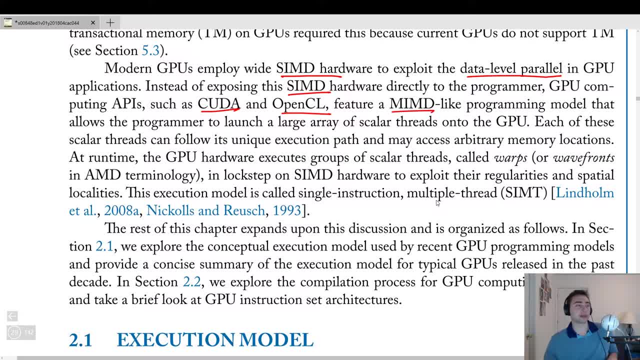 and CL. They feature a MIMD-like programming model that allows the programmers to launch a large array of scalar threads onto the GPU. So each of these scalar threads- because MIMD stands for multiple instruction, multiple data and these things are again- are scalar threads. 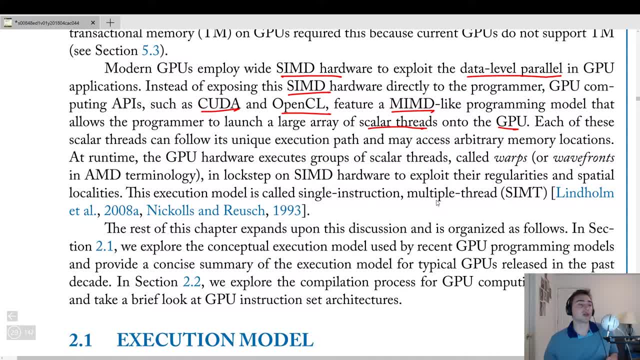 So each of these scalar threads has the ability to follow a unique execution path, So every single thread could be doing its own thing. We could have this big if-else-if-else-if-else-if statement and kind of section off threads one by one, and every thread could do something different. 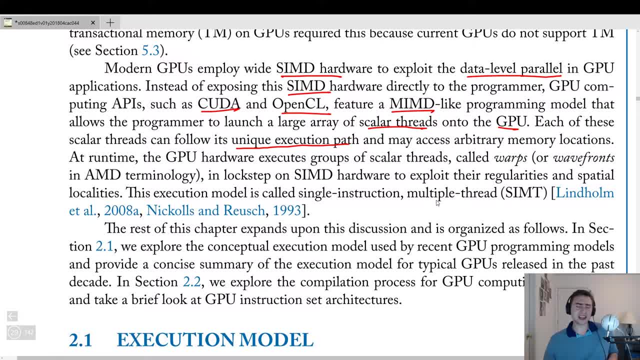 But it's important to note that at runtime that's not exactly how things get executed. So these scalar threads aren't just completely independent and, you know, individually schedulable, They're actually grouped into things that NVIDIA calls warps and AMD calls wavefronts. 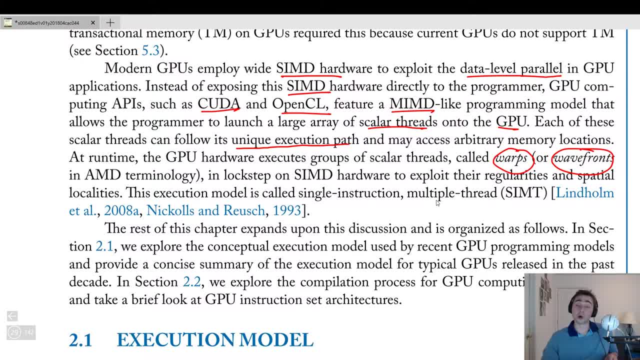 So these are just collections of things that we can do. In the case of warps, 32 threads and in the case of wavefronts, 64 threads that operate in lockstep. So this means that every single thread is doing the same operation at the 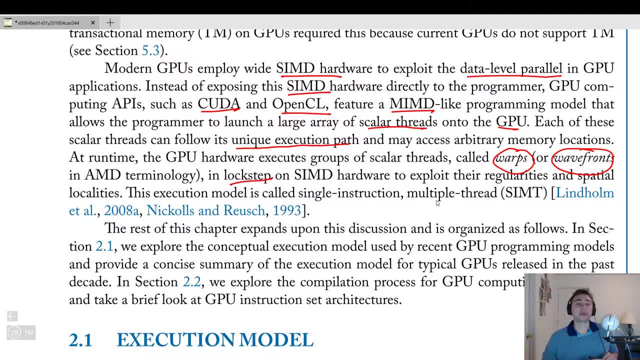 same time. So if we have, you know, an add, all 32 threads in a warp will all be doing an add. So we'll only have one instruction, And this execution model is called SIMT. so we'll have this, you know, this vision of scalar threads, Even under a SIMT model. we just have to. 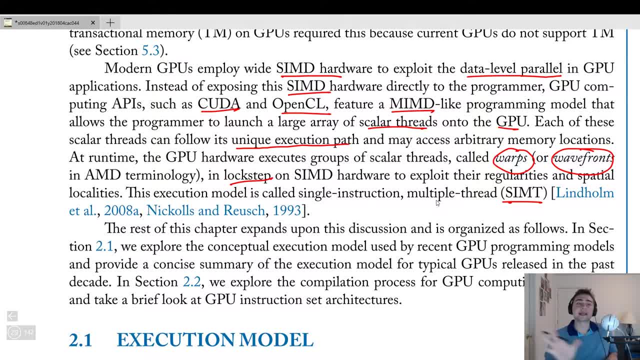 make sure that we have something called an active mask which says which threads inside of a warp are active at one time. But in reality, when we're programming these things, we really should be thinking about what entire warps are doing at the same time and avoiding having you know. 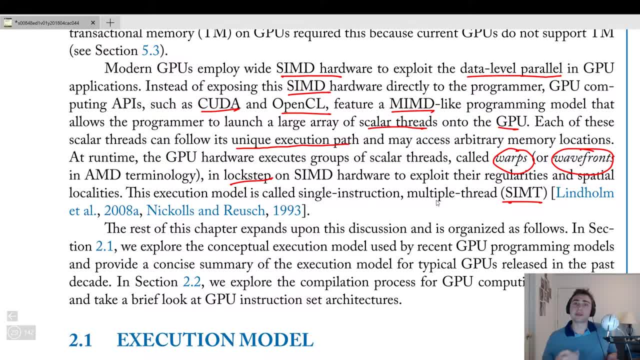 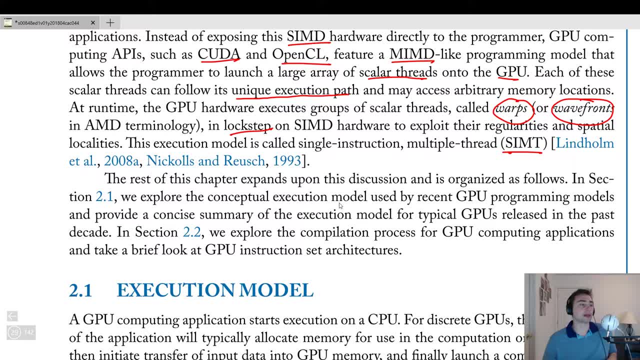 every single thread in a warp be doing different things, which is something that we call warp divergence. But we'll discuss that later on and how that works. So let's go ahead and get started with the execution model. So again, kind of like we saw. 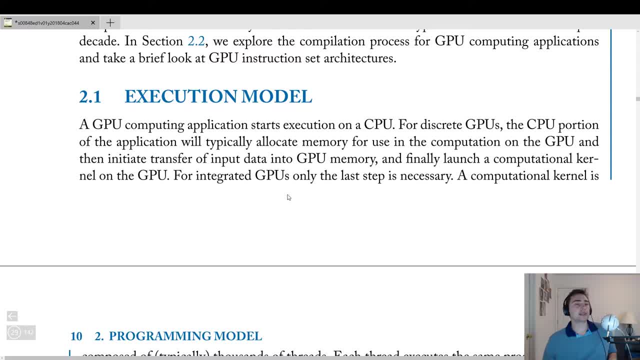 in the previous chapter. So everything starts really with the CPU. So the CPU is kind of the thing that kicks off everything when we're executing GPU code. So typically from the GPU we'll allocate memory right, So we'll do something like a CUDA malloc, So just like. 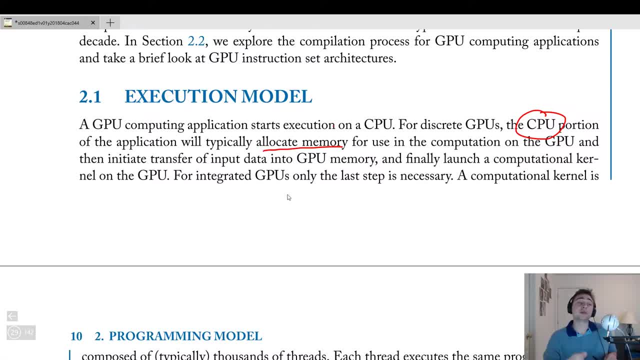 malware, So we'll do something like a CUDA malloc. So we'll do something like a CUDA malloc. It'll allocate some memory For the CPU. CUDA malloc allocates memory on the GPU, So a lot of times when we're programming these things, we have a discrete GPU, So it has its own memory, So we 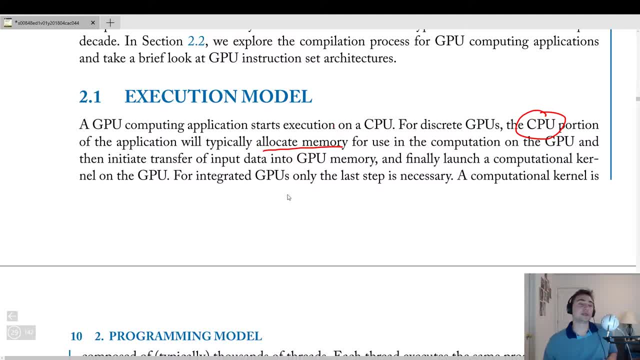 have to call CUDA malloc In the case. this is of course in the case for NVIDIA GPUs. you know OpenCL does not have CUDA malloc. And then of course, there'll be a data transfer. So because the memory is separate physically, we have to copy the memory from CPU memory all the way to GPU. 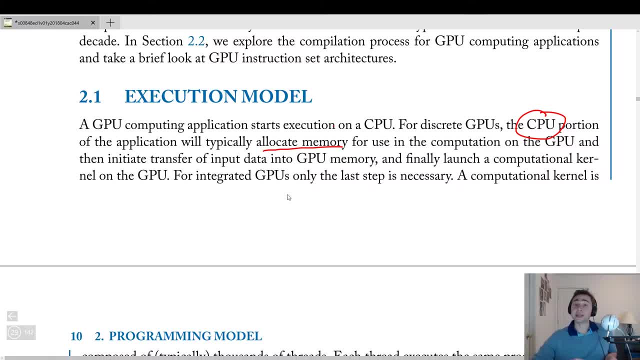 memory. So we have to copy the memory from CPU memory all the way to GPU memory, And then, of course, there'll be a data transfer from CPU memory all the way to GPU memory, And this is typically done with a function call. In the case of NVIDIA, this is CUDA memcopy, So fairly straightforward. 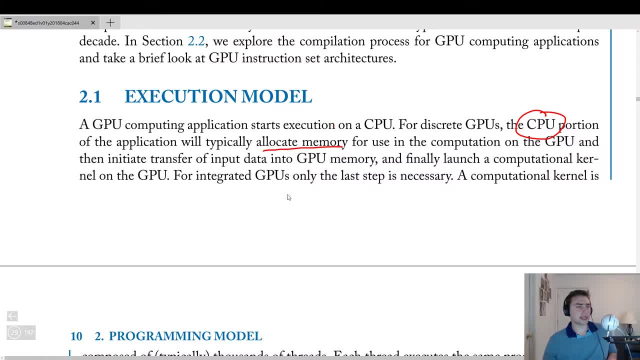 name: Okay. So again, this transfers our input data to GPU memory And then we'll launch, right? So then we have to tell the GPU: hey, I have a kernel for you to work on. Here's the kernel, So for. 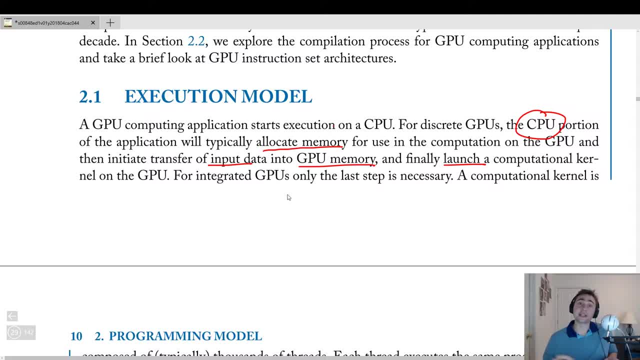 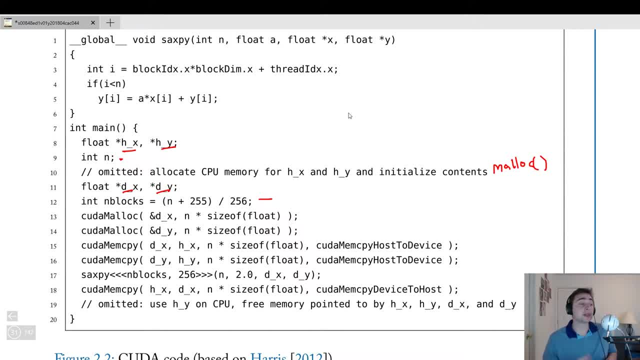 So this is something that we can't dereference on the CPU. This is something that's only valid on the GPU, because it's completely separate address spaces, because it's completely separate memory, right? Then, of course, we'll have to copy the data over. 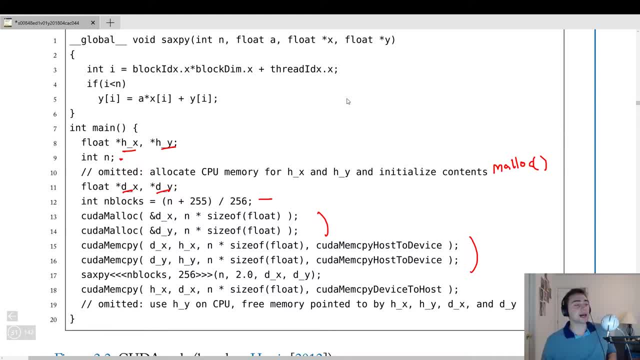 And so we use CUDA memcpy for this. And so we say: I want you to put into this DX, which is our pointer to device memory that we allocated here. I want you to put whatever is in H of X, So that's our host memory. 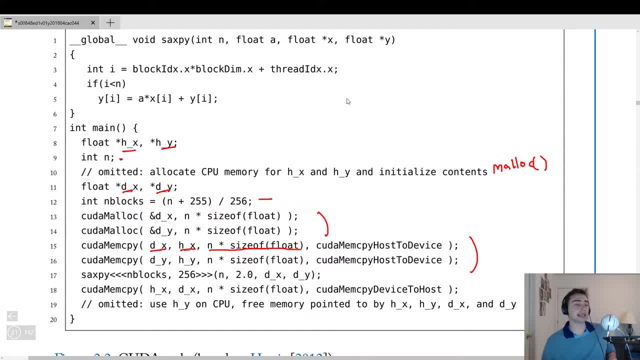 Then, however many bytes, in this case is just going to be n, which is the size of our array times the size of a float right. So it's going to be, you know, four bytes times the number of elements in the array. 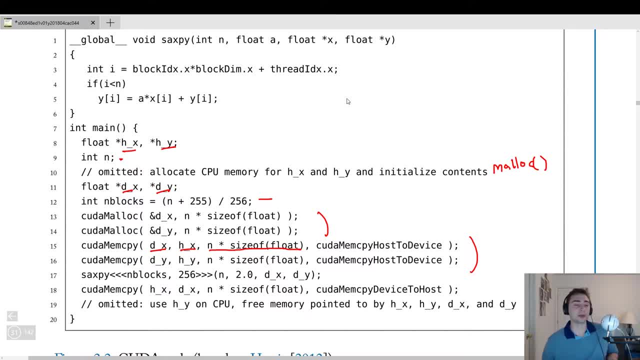 And then we have to specify a direction. So we'll specify CUDA, memcpy, host to device. If you want to copy things back as we see down here, it's a copy them back. You know this will be to GPU And this will be from the GPU. 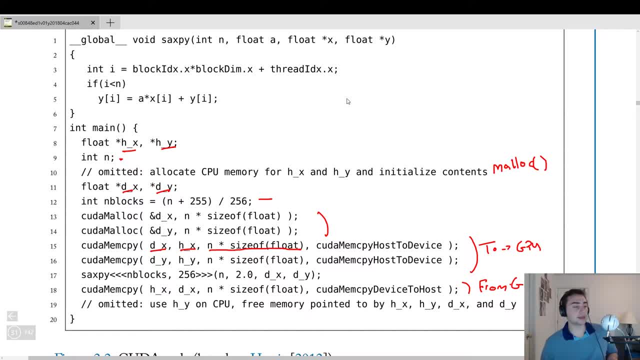 And so it's pretty similar in this way. The only difference is our target is first, of course, So our target was the device side here. So here the target is going to be a host pointer from a device pointer. Then it will be n times size of float. 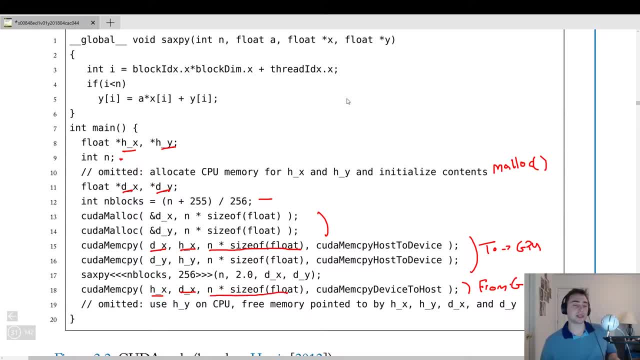 So this is just, It's the number of bytes, And then we specify the opposite direction, So instead of host to device, it becomes device to host, And then of course we do some free over here, right, So we'd free our host memory. 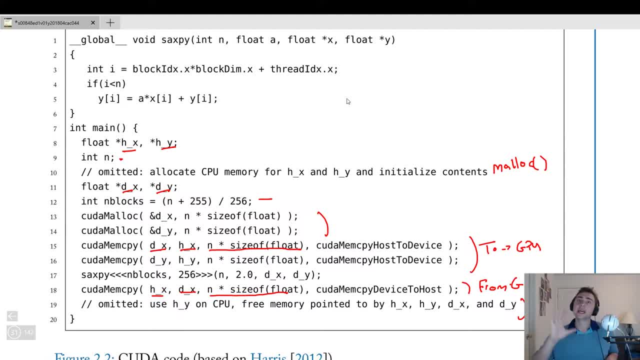 And then we'd also do CUDA free, which is just the same thing, except it frees device memory. So now let's talk about, you know, the little bit nastier parts of GPU programming that we skipped over. So, as we mentioned in the last video, 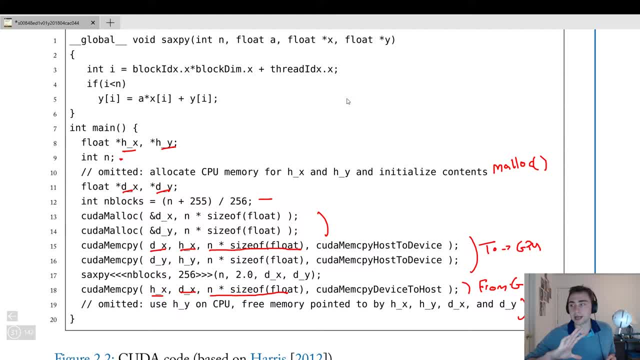 in order to, you know, get this parallelism, we have to set up a grid of threads that we're going to launch, right, And so that's our grid of scalar threads, And so programmers define this in really two different ways. 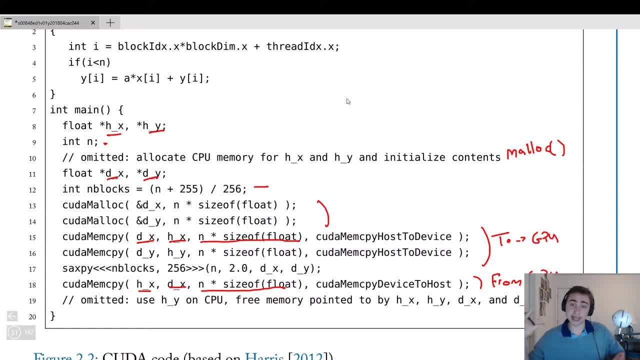 So they define it as an entire grid and then they define it at chunks of the grid, called thread blocks, And so let's do a very simple example here. So let's say I want to launch four threads. right, I have four scalar threads here. 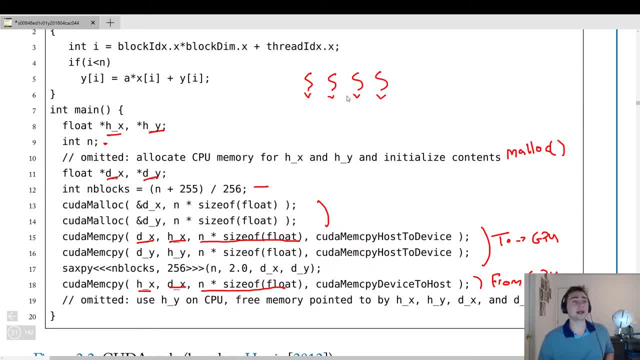 that I want to launch. Well, eventually, as we scale this up and up and up, we get a limitation on, you know, the number of threads that we can launch inside of a schedulable thing called a thread block. So if we put everything in one thread, block right. 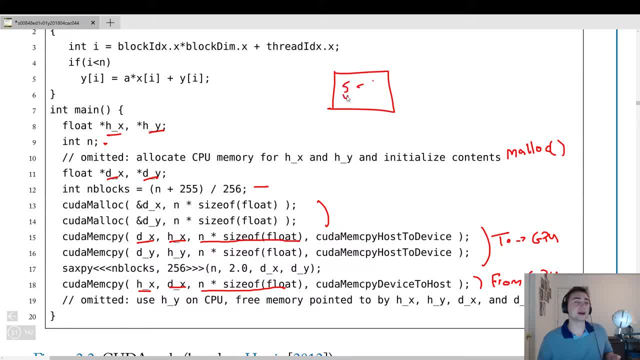 So you can think of having this thread block. It has some number of threads in it. Eventually, you know, this thread block will get full. There's dimension, There's constraints on a thread block And thread blocks are the things that actually 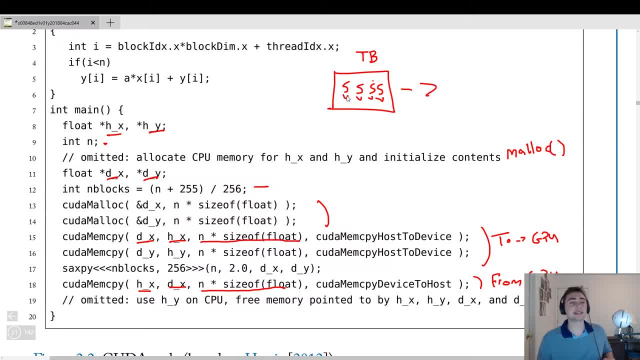 So we'll call this a TB for thread block, And this will actually get scheduled to an SM, so a streaming multiprocessor, which is just a core. So what we want to do is we want to put all of our threads into different. 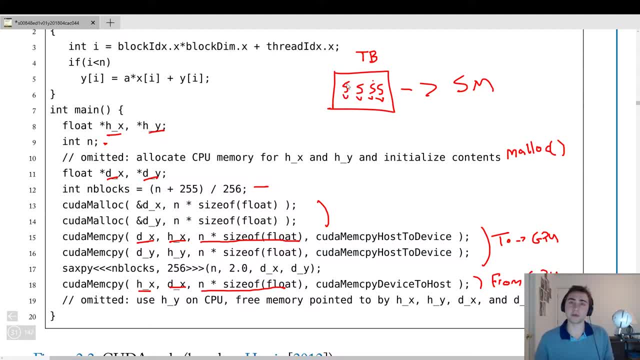 We want to have groups of threads inside of thread blocks. We want to launch multiple of these things so they get spread out across all the cores. So let's do a simple example: where we have, We have a thread block that can hold two threads, right. 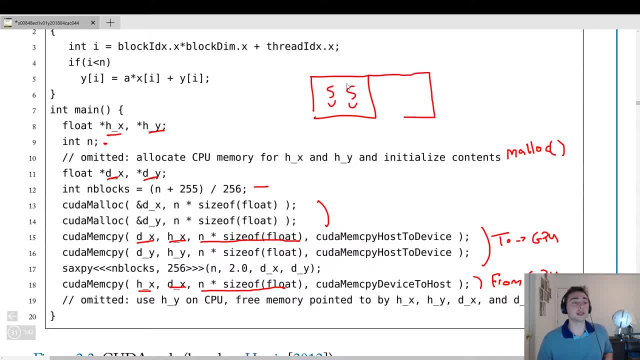 And then say: if we want to launch four threads, we'd launch two thread blocks. If we wanted to launch six threads, we'd launch three thread blocks, right? So this is just a very simple example. In reality, we can launch a lot more threads. 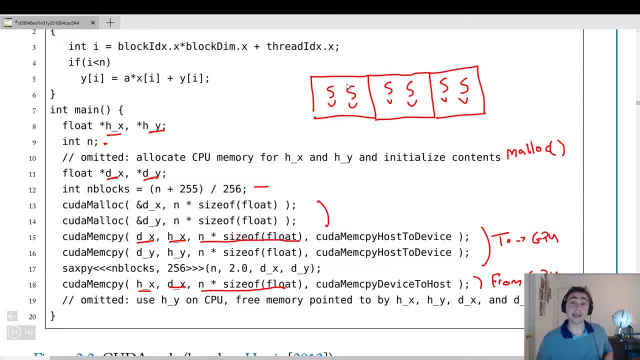 per thread block than this. And again, you know we talked about warps earlier and wavefronts. The programmer doesn't actually. He doesn't actually see warps and wavefronts, So thread blocks actually get decomposed into warps and wavefronts behind the scene. 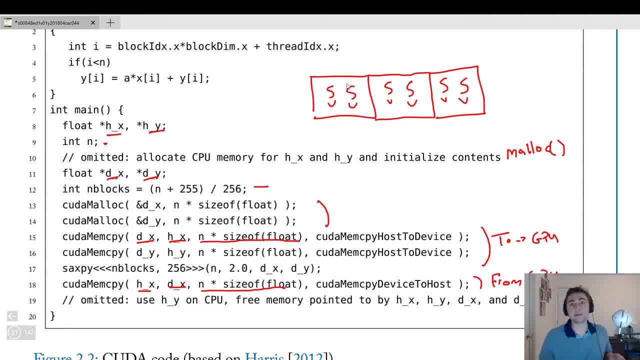 All the programmer sees is thread blocks and a grid. So each of these things is a thread block, And then the collection of all of these thread blocks is a grid, right, So it's a grid of thread blocks, Okay, So let's get rid of this. 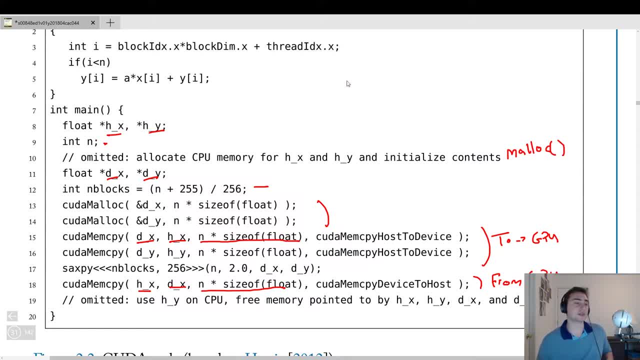 And then let's get to the A little more complicated parts of GP programming. So let's start here. So the number of thread blocks that we want to launch, We specify that right here, And in this case it's n plus 255 divided by 256.. 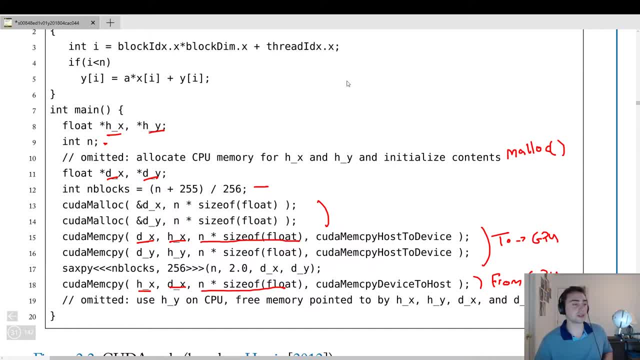 So this is a little non-intuitive when we first look at it. So I'll break it down of what they're trying to say here. So one of the assumptions being made here is in the kernel launch itself, which we'll get into in a little bit. 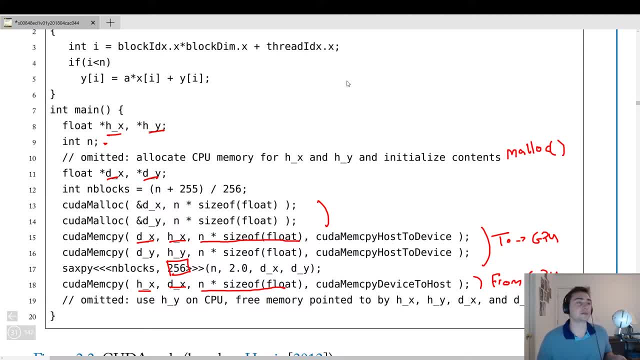 So for a kernel launch, we specify two things. We specify: We specify a grid size and a block size. Block is just short for a thread block, So we can say a TB size, right. So we specify how many blocks we want to launch. 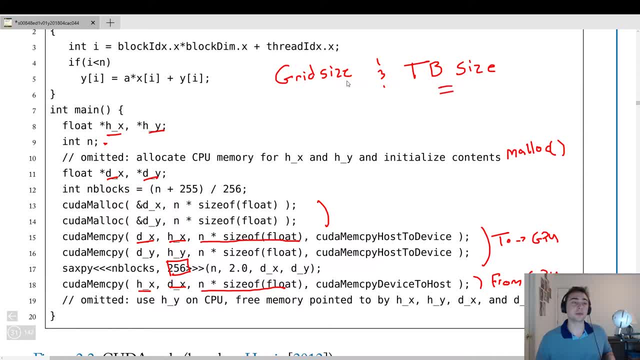 And then this is equivalent to how many threads per block. So down here, that's the order here. So the number of blocks, This is the grid size, And the threads per block is 256.. So that's where this 256 comes from, as well as this 255.. 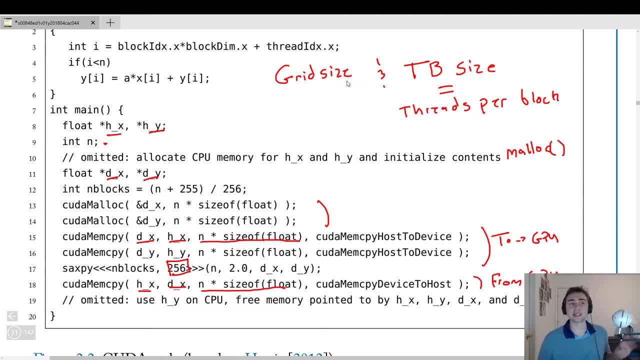 This comes from this assumption that they're launching 256 threads per thread block, And so in the example we looked at, we just had two threads per thread block. So let's see where this n plus 255 comes from. So sometimes we get really lucky. 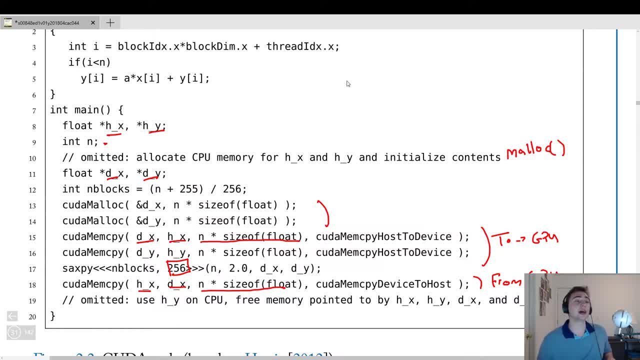 and we have input sizes that are a power of two. Other times we're not so lucky. Maybe we'll get an input size of 1,000 instead of 1024. And so we have to be able to pad those empty threads. 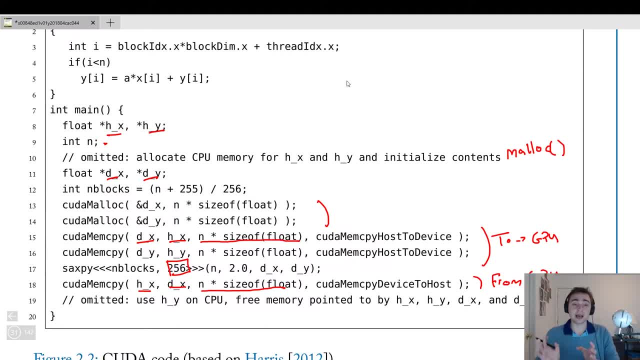 in a thread block, to make sure that you know, even if every thread in a thread block isn't working, we're still calculating the entire operation of, say, Saxby. So let's see where this n plus 255, dot 256 comes from. 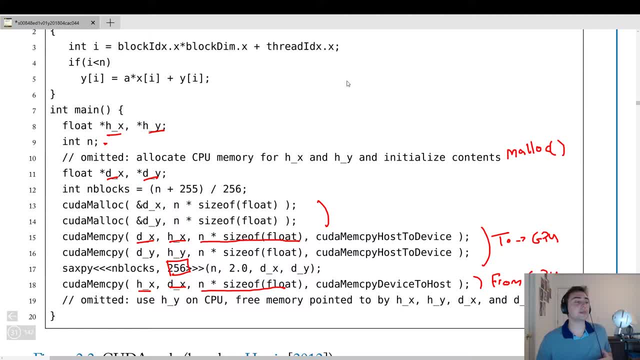 So let's say we have our thread blocks that are size two again And we have a problem size that is say, you know, n is equal to 5. So in this case, how many thread blocks do we need to launch? 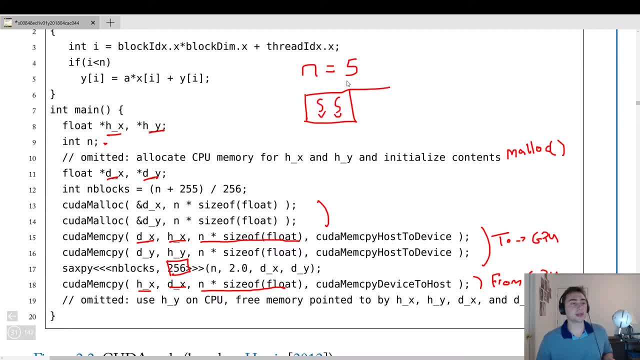 So here's a thread block with two threads. Here's a thread block with two threads, And then here's our final one. Now, all the thread blocks have to have the same size, right? So we can't have one with less threads. 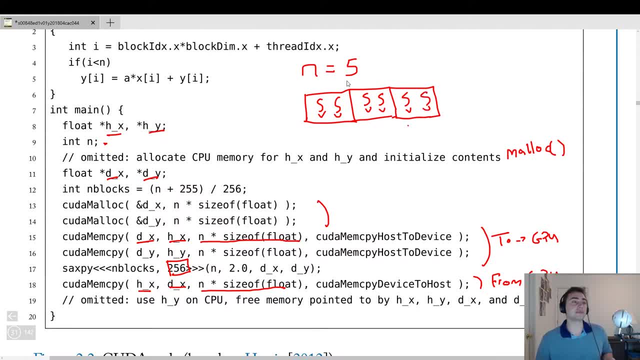 So we have to have two threads here, right? Even though we only have five elements. So how do we get from five to three thread blocks? So we have to do some padding- Padding, right. So that's where this n plus 255 comes from. 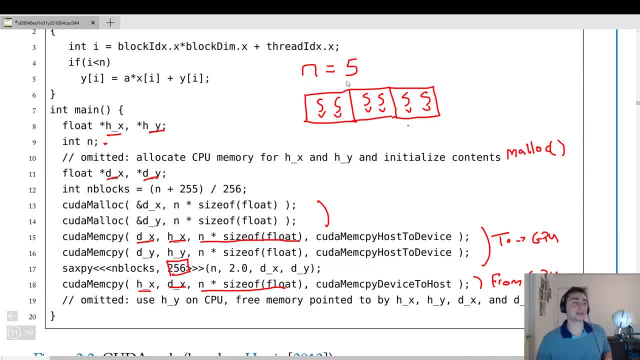 So if instead this was two threads, this would be n plus two minus one, right? So over here is the number of threads minus one divided by the thread block size two. So in this case it's just padding to make sure you get to the 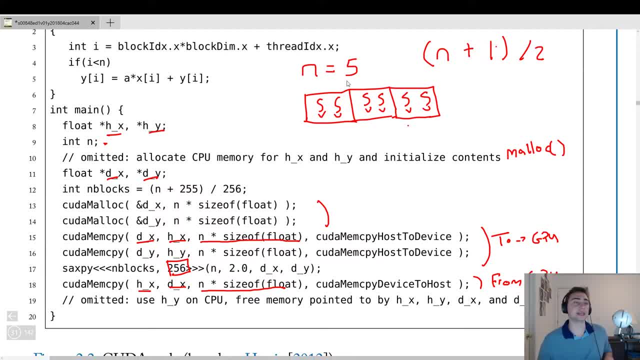 at least to the very end. right, Right, Right, Right, Right, Right Right Of a thread, block right. So n plus one divided by two is going to, in this case, be five plus one divided by two. 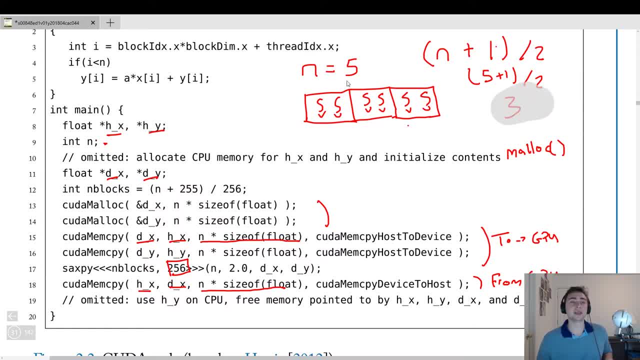 which is going to be equal to three right, So three thread blocks. If we didn't do this padding at the very end, what would we wind up with, Say, if we just want to split our problem by dividing the total number of elements? 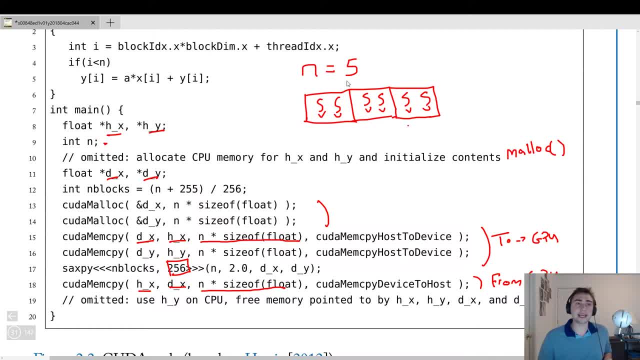 by the number of threads per thread block. Well then, in this case we would do five divided by two. So we would do five divided by two, which is going to equal 2.5,. right Now, the thing is, this is an integer right. 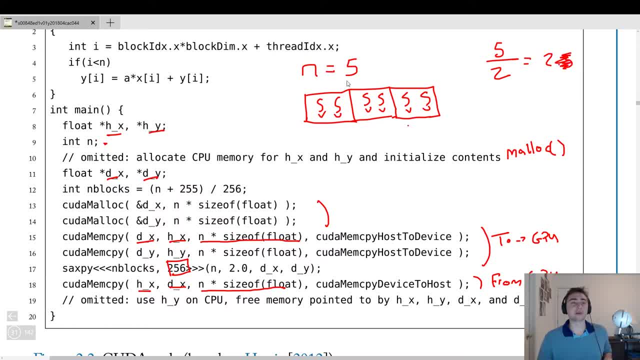 So it's int num blocks. So we won't keep this 0.5 part, So we'll only launch two thread blocks And then the last element of these vectors won't get calculated. So we have to make sure we do this padding. 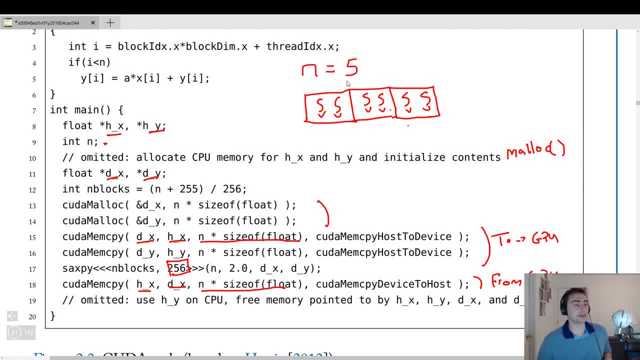 especially if we're doing, you know, if we're calculating things that aren't a multiple of, you know, the threads per thread block. If everything was a multiple, if it was a multiple of 256, you know it would always divide evenly. 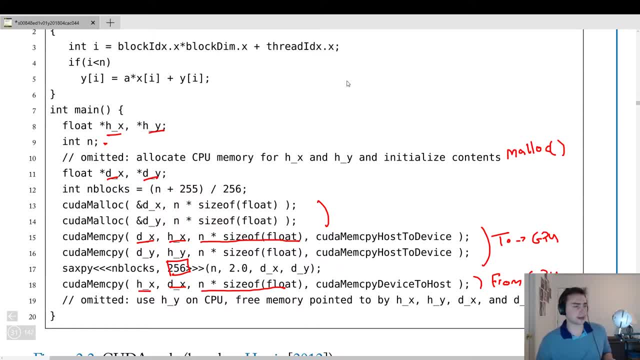 So we have to do a little bit of padding. So that's kind of the basics there. So over here we calculate our grid size. So in blocks is our grid size. So this says that in the case of our simple example it would have said we were going to launch three thread blocks. 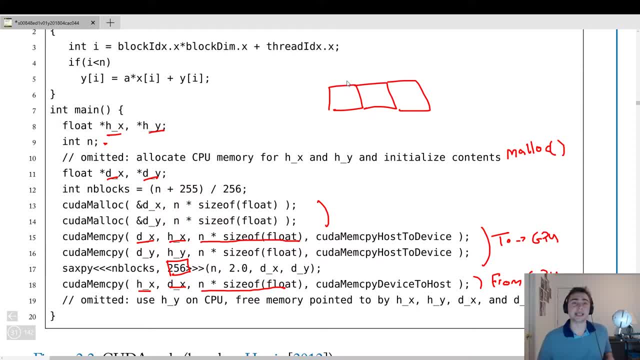 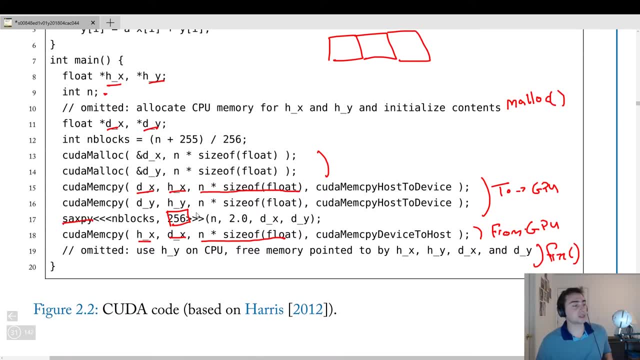 In this example it's kind of generic because we don't specify what in is. And then down here is where we actually launch the kernel. So we have a kernel called Saxby. We're going to launch a grid size of some number of blocks. 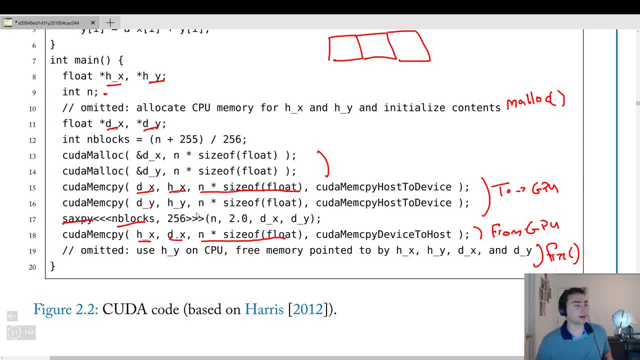 And we're going to launch some number of threads here, In this case 256 threads per thread block. Again, this is per thread block, And then we'll have some parameters here And notice that we put all of these block and grid dimensions. 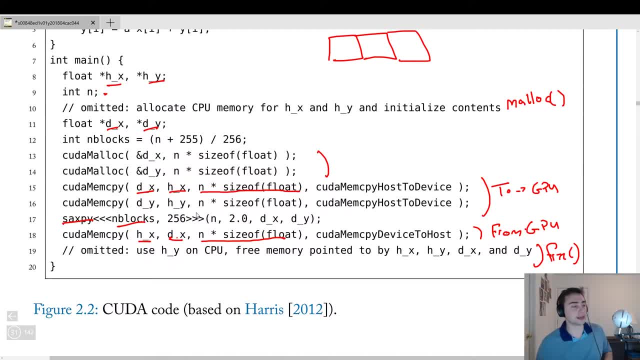 inside of this kind of triple less than greater than sign notation. So it's kind of funky This kind of triple chevron notation. But somebody decided that's how we want to launch kernel, So that's how it happens. So that's kind of our setup. 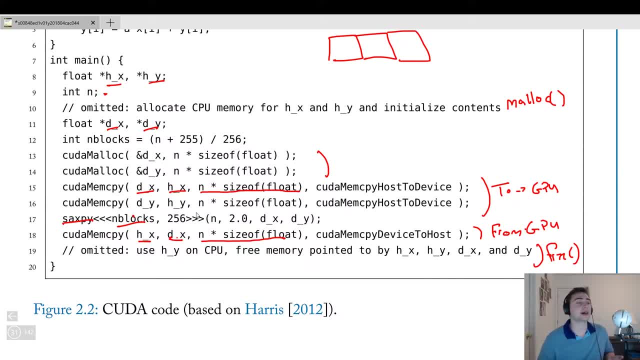 So now we know how to kind of define a grid, We know how to define the number of threads we're launching overall, We know how to allocate memory on the GPU. We know how to copy memory onto the GPU. So what's left? 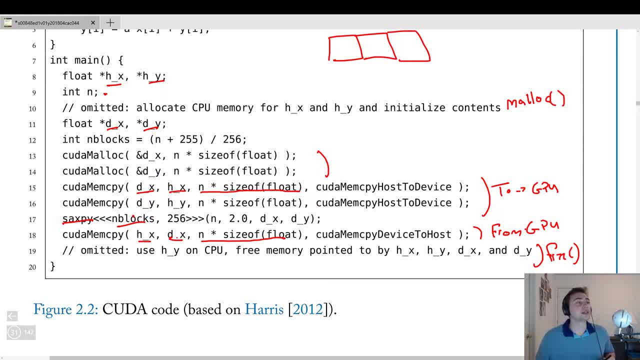 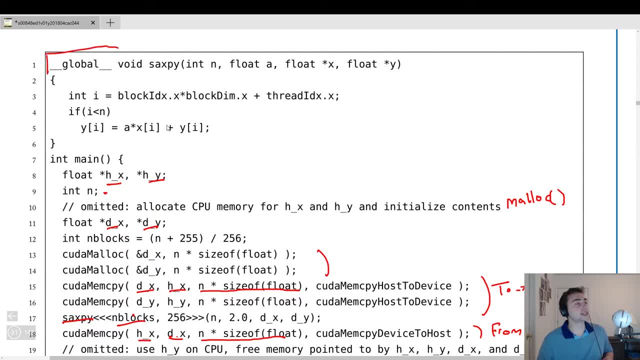 Well, of course, the actual kernel itself. So now let's look at the kernel. All right, So here we have it. We always specify in CUDA a kernel. We'll start with this global right here. So this just says I'm a function that will be executed on the GPU. 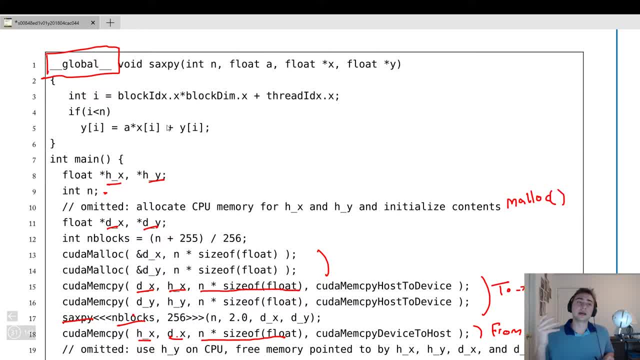 and I will be called on the CPU, So the CPU will call this function and then tell the GPU to do this work. There's also this: This could also be device And that's a special kind of, you know, a function. 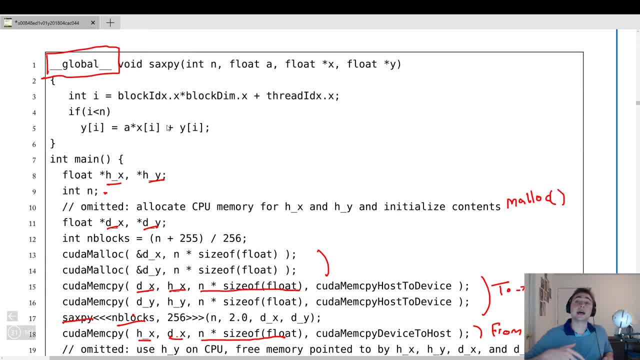 which is called a device function, And that is something that it doesn't start on the GPU, or sorry, it doesn't start on the CPU. It's a function that's called directly from the GPU, But we'll leave that to another time as well. 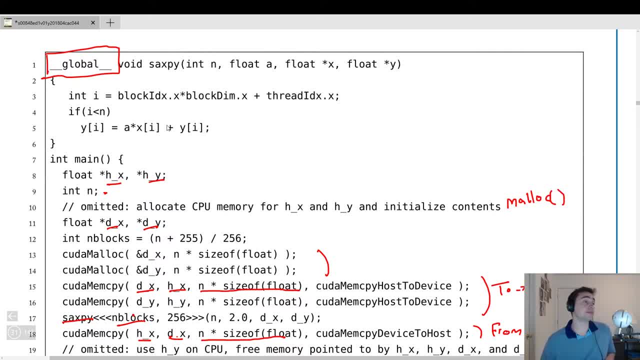 So the rest of it is exactly the same, as it's exactly the same as a normal function You would see in C or C++. You know it's just a void function called Saxby. You know it takes some parameters. In this case it'll take an integer in. 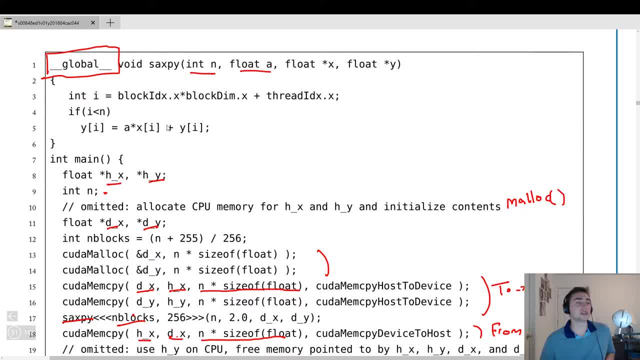 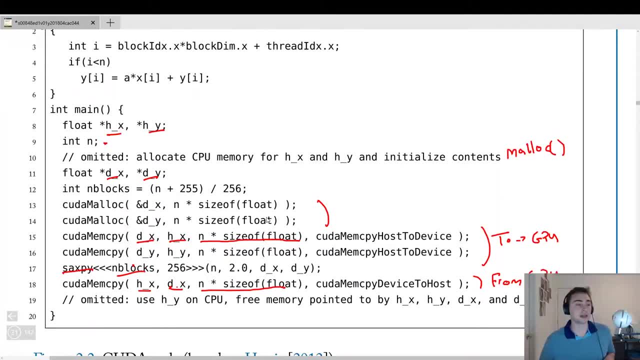 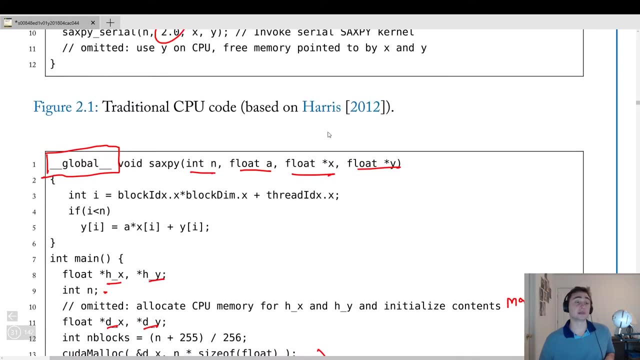 So the number of elements, A, float, a, Which is just how we're scaling. And then two pointers to device memory. Remember down here, when we call the function, we pass it the pointers that we allocated with CUDA, malloc, right, We don't pass the host ones because you know, on the GPU, 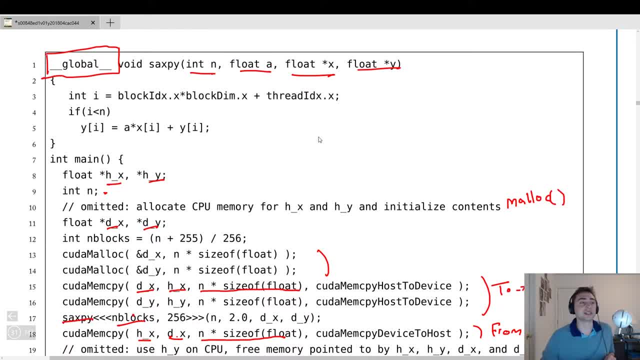 you don't understand CPU memory if you're on the GPU for discrete devices, So it has to be the device pointers. Okay, So then we have our first kind of new line compared to the last one, which is this: block IDX, block dim X and thread IDX. 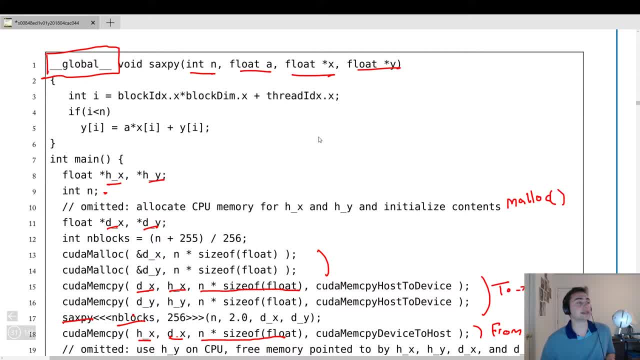 And then it's this int: I is set equal to that. So all of these values are things that are kind of they're built in values for every single thread. So, as you can imagine, it's important that every thread knows where it is within our grid of threads. 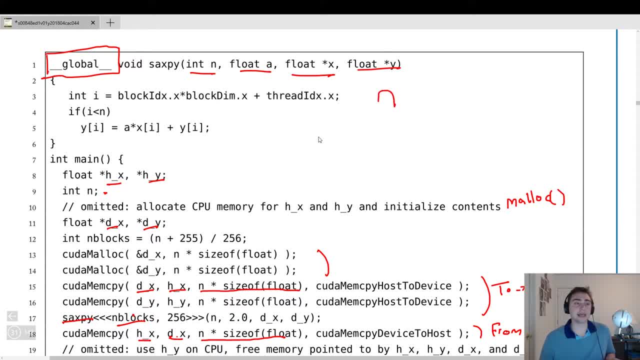 So let's get back to our simple example of, say, you know, in is equal to five And our thread block size, You know, TB size is equal to two. So there's two threads per thread block. So here we have you know, two threads in the first thread block. 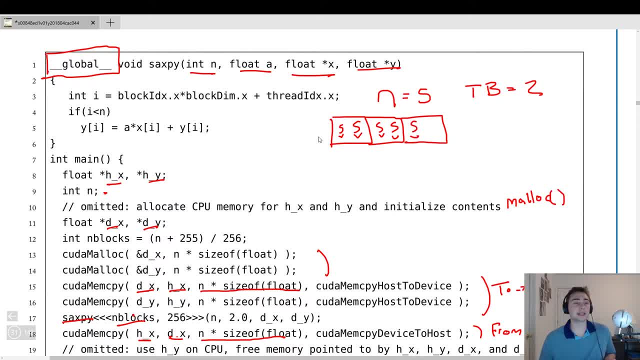 two threads in the second thread block and we have two threads in the last thread block because they all have the same number of threads. But this thread is actually not going to do anything right? So this thread is just kind of it'll be idle. 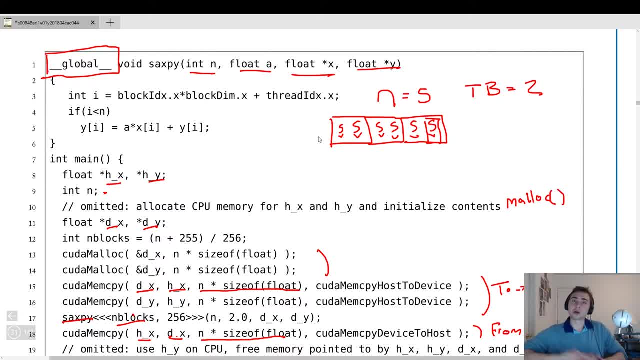 So you know how do we figure out which thread we are globally in the entire system. So we know that this thread should access element zero. This thread should access element one on. this thread should access element four right. So intuitively that makes sense. 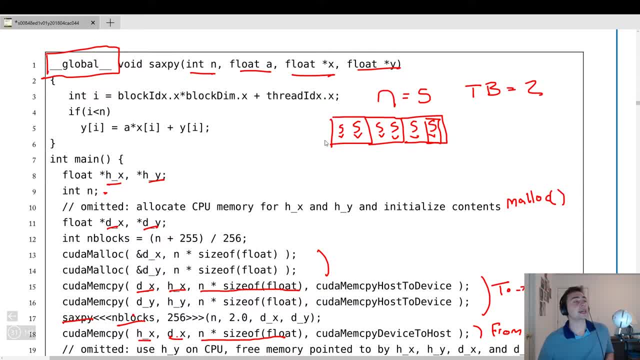 But how do we get to you know, how do we tell the threads that? And we do it through these variables right here. So we have a block ID, a block dim and a thread ID. So a block ID is just going to be which thread in a specific dimension you are. 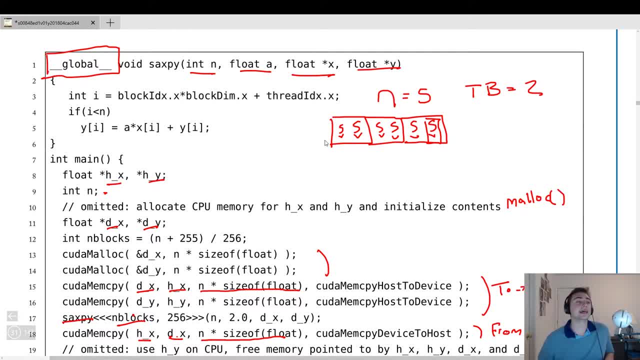 So one thing that I kind of omitted is that you know grids and blocks can have, you know, parallelism defined in three dimensions. So I could have blocks defined in the x dimension, the y dimension and the z dimension And I could arrange threads within a thread block into an x dimension, a y dimension and a z dimension. 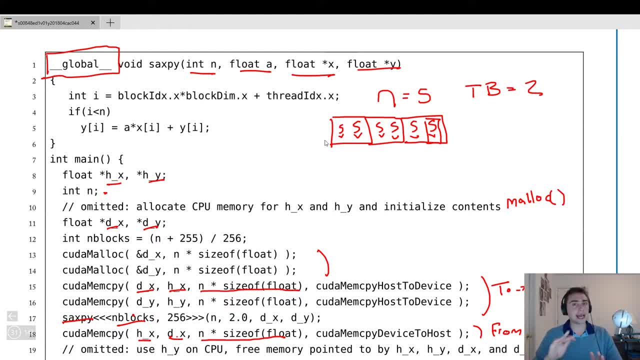 For something as simple as this. we don't need that extra, those extra dimensions. We just have a big, long, you know array. So all we need is a single x dimension. So we'll kind of ignore that other, that other dimensionality for now. 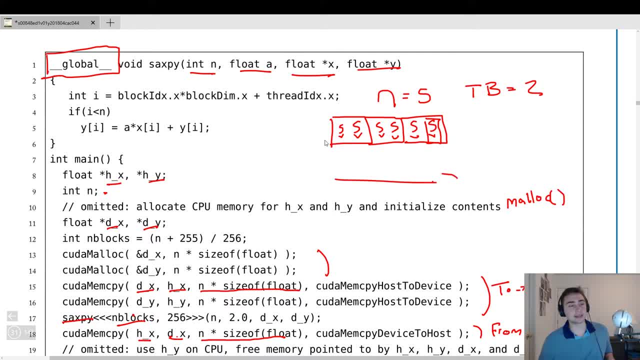 So again. so if we consider this to be the x dimension, So let's look at the block ID. So this will have block ID zero, This will have block ID one and this will have block ID two. right, So they just, it just linearly increases. 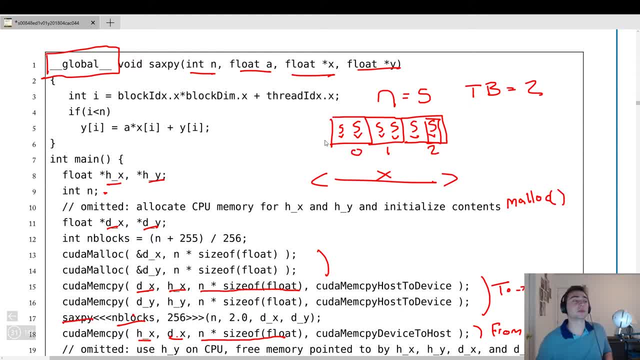 And then the block dimension. this is going to be the same for every single block And that's just the number of threads that are in the x dimension For every single block, When in this case it's going to be two. Every thread has two thread blocks in the x dimension. 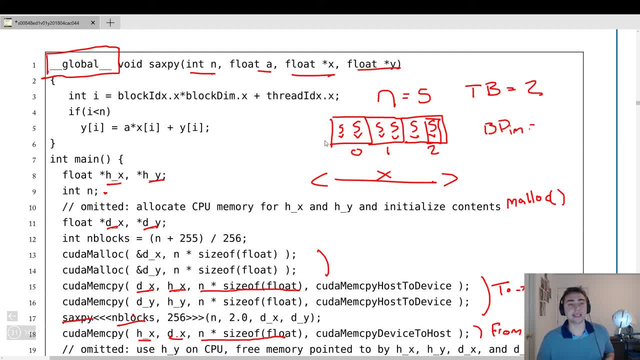 So you know. so we can say: bdim is equal to two. And then of course we have thread ID x, dot x, Which says which thread am I in the x dimension in this particular block Right? So here we'll have thread zero. 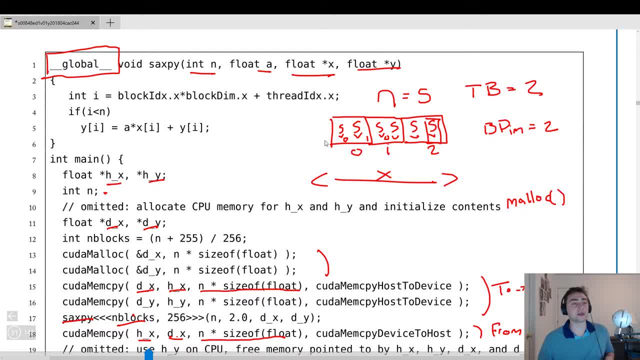 Here we'll have thread one, Here we'll have thread zero, Here we'll have thread one, And this will continue on. So how does this calculation look like for a particular thread? So it's a very simply a base offset, right? 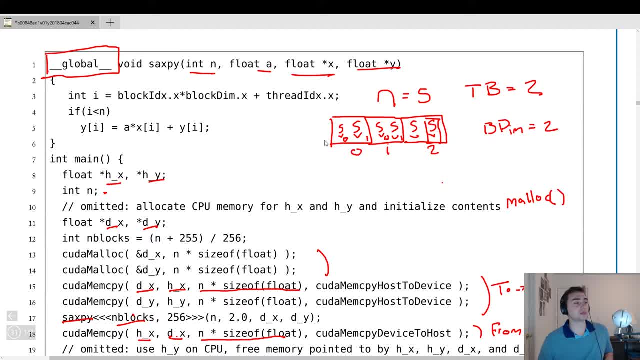 So to figure out the base, we calculate this block ID x times block dim x. So if I'm block zero, this base will be zero. If I'm block one, this base will be two, So it'll be block ID x one. 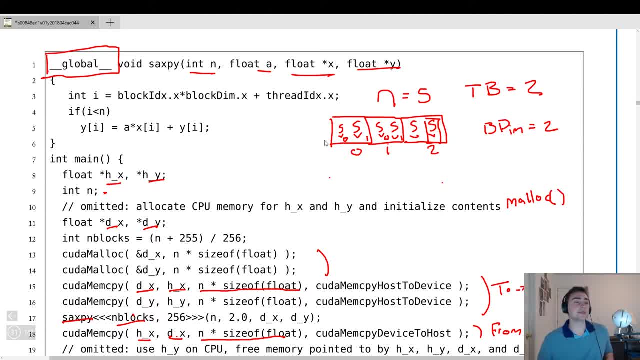 Times block dim two. And then, if I'm in the third block, my base will start at four Right. So it'll be block ID x, which is two Times block dim x, which is two Right. So this is four. 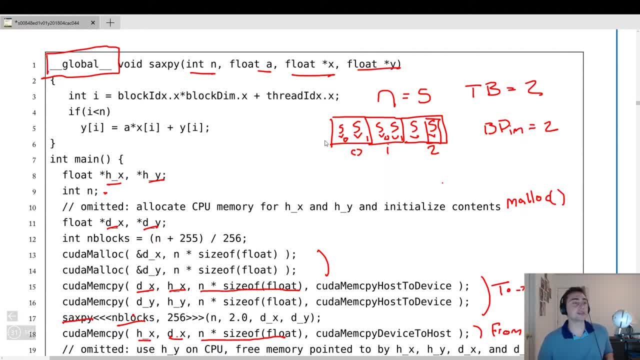 And then we find so that's our base And then our offset is just going to be the thread within that block. So if we take something in the middle here, So let's say we want this thread right here, Right, So our block ID x is going to be one. 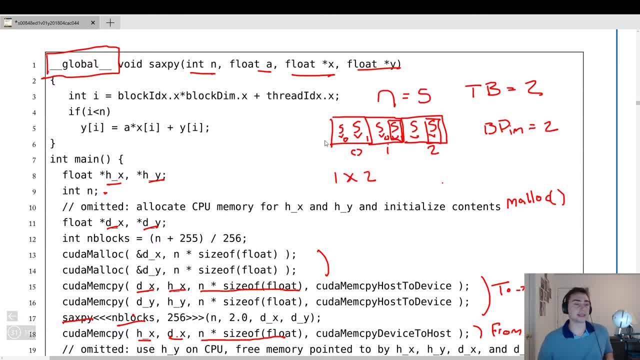 Our block dim x is going to be two- Remember that's the same for every block- And then our thread ID x is going to be. so this is thread zero, this is thread one. So they literally increase from zero to however many threads you have per thread block. 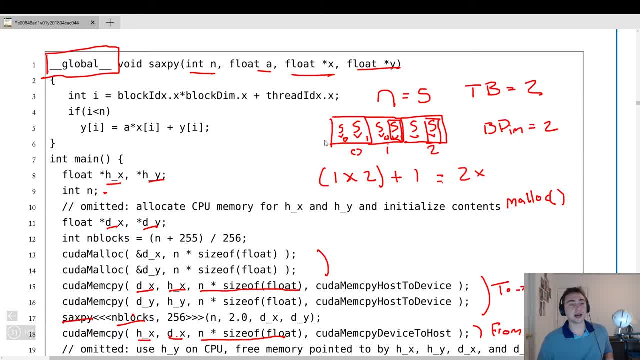 And in this case it's going to be one. So this will be two times one plus one, which is equal to three Right, So, and that makes sense if we were to count linearly up from starting from the first thread. 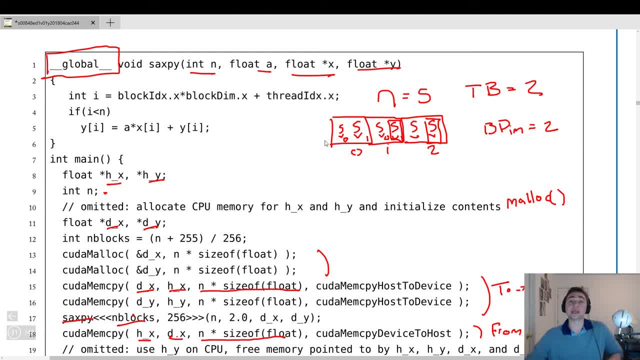 So this would be zero, one, two, three Right. So, like I said, this calculation is just finding a global thread index. So which thread am I with respect to the entire grid? And so it's fairly simple in this case. 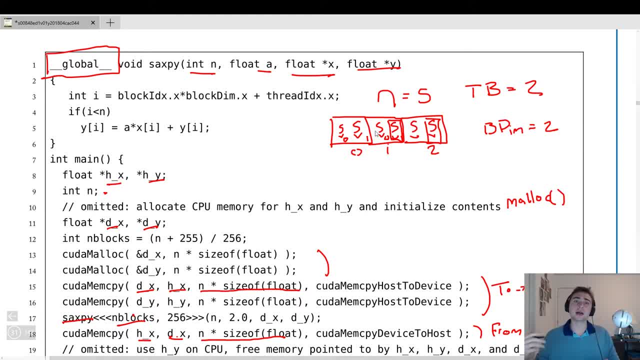 Once we start doing two-dimensional threads- like I have in the CUDA crash course videos for handling, say, a 2D matrix- You know we have to both calculate. you know a row and a column, But in this case it's fairly simple. 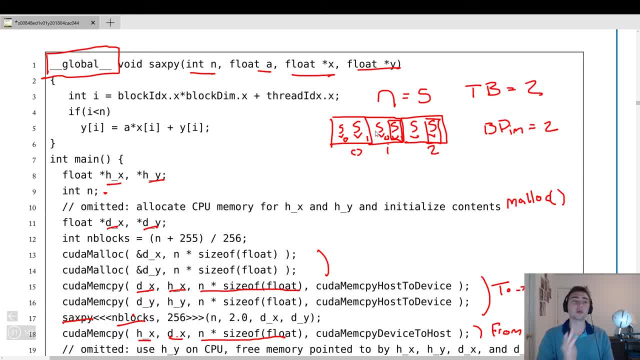 It's just one dimension. We just have a big long line of threads and we need to figure out where we are in that line. So then we have a simple comparison statement. So we want to make sure that, you know, is the thread that we launched? is it active? 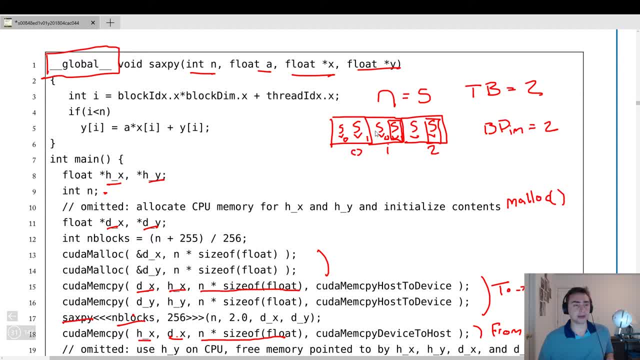 Right, So in this case, in our simple case, right here. so let's clean this up a bit. Let's draw this again. So we launched three thread blocks, But our last one had an inactive thread in it. Right, So we had these five, because n is equal to five. 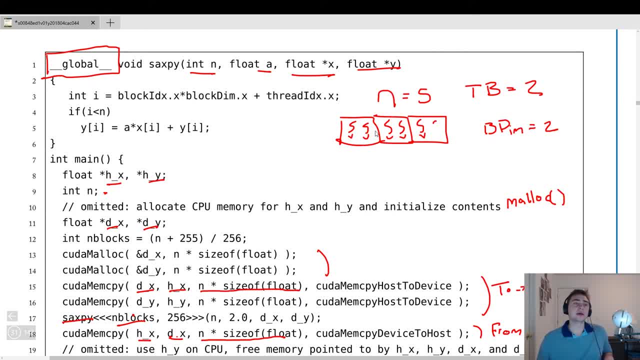 That's the number of elements. So we want to launch as many threads as elements. But we had to do a little bit of padding for this last thread because we have to launch a fixed size number of thread blocks, Or rather the number of thread blocks have a or the thread blocks themselves have a fixed size. 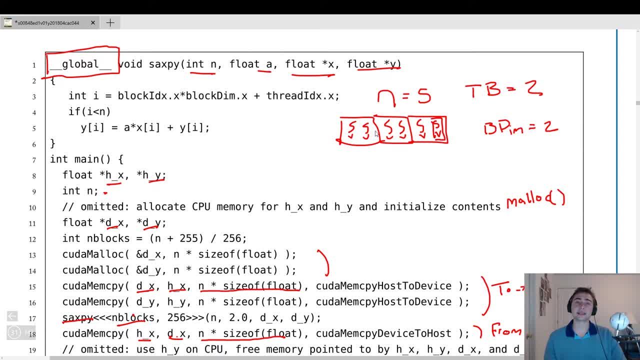 So how do we avoid this thread doing anything nasty? Right? We don't want him to access memory that's out of range. We don't want him to interfere with anyone else's memory. So it turns out we can just do a simple comparison. 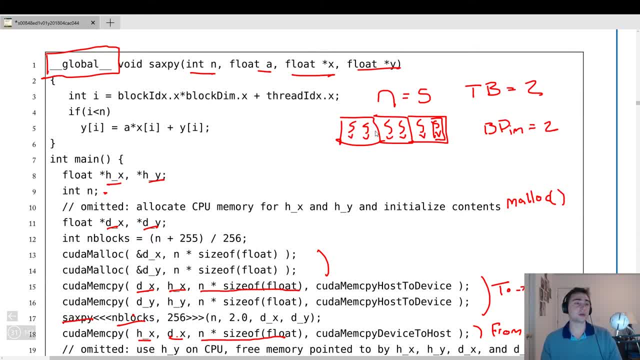 So we just said: if i is less than n right, So this thread, this calculation, i will be zero. This will be one, two, three, four, five. So this one five, our n, is equal to five itself that we pass in right here. 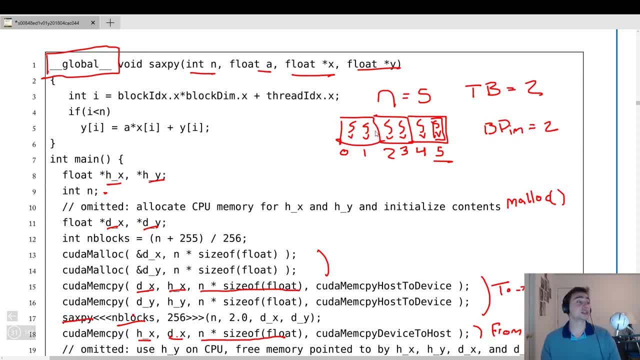 So in this case five is not less than five. So it just doesn't do Saxby, It just doesn't do a times x plus y. So you know, we launched a thread, You know the thread's not doing anything. 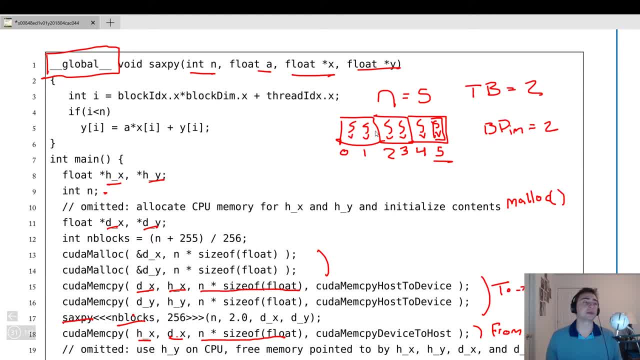 But that means it's also not harming anything. So we can get away with that Right, And sometimes we have to do that if we have an awkwardly sized problem, And so that's kind of the basics of the GPU kernel right here. 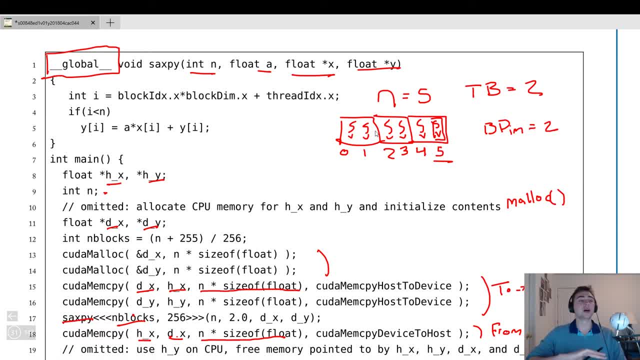 So the general process that we do is, at the very beginning of the kernel, we'll, you know, figure out what position you know a thread is in with respect to the entire grid, And then we'll start doing computation based upon its position in the grid. 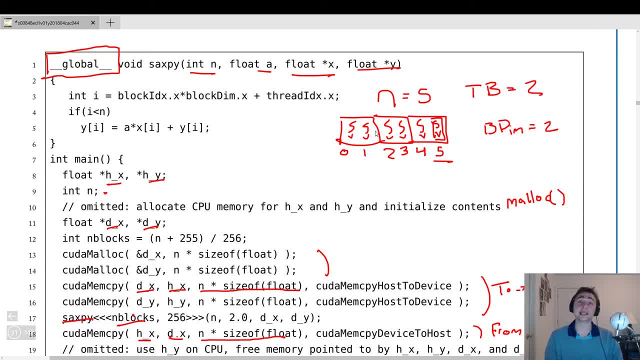 So, again you know, instead of having a for loop here, like we had in the serial Saxby, that for loop is replaced by just a calculation of a position in a grid Right. So that's what's used to index y and x. 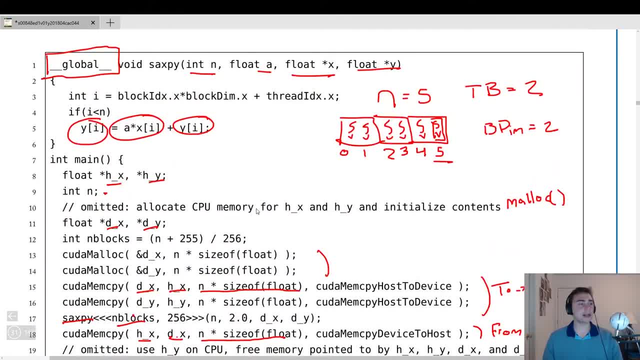 Okay, So a little bit complicated, But Fundamentally it's the same. We just need to figure out We're basically unrolling a loop, So every iteration of the loop now just becomes the operations of a different thread. Okay, 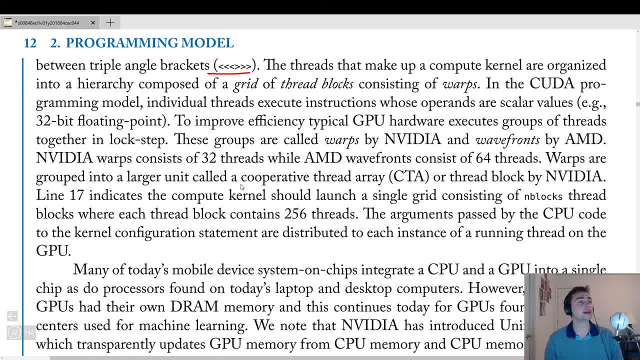 So some cleanup stuff. Let's talk about some basic things. So again, these triple angle brackets is what we use to define a grid of thread blocks And then, behind the scenes, this will get translated back into warps or, in the case of AMD, wavefronts. 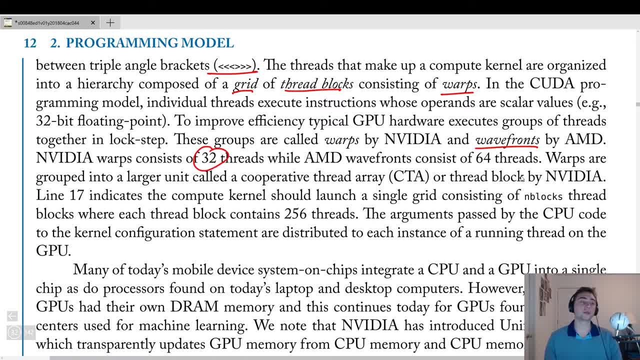 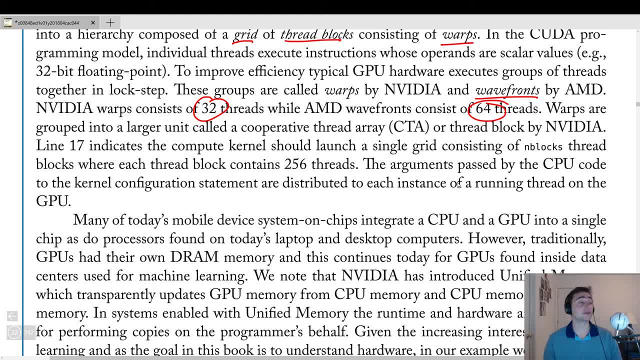 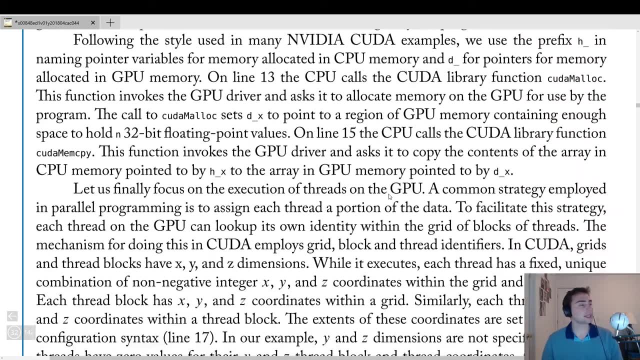 Again, NVIDIA has. NVIDIA has size: 32 warps, while AMD wavefronts consists of 64 warps. Occasionally, thread blocks themselves will go by a different name. Sometimes people will call them a CTA or a cooperative thread array. Let's see if there's anything else. 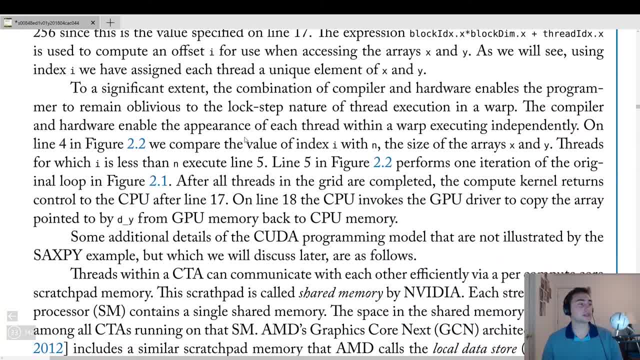 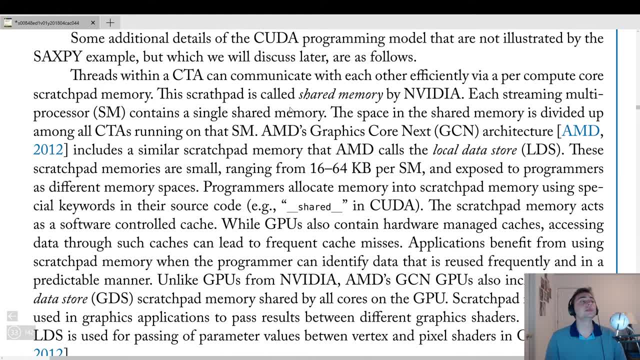 I think that's going to be about it. So there's some other things that we can do as well. So inside of, We can do a little bit of optimization. We can do a little bit of optimization inside of the GPUs themselves. when it comes to programming, 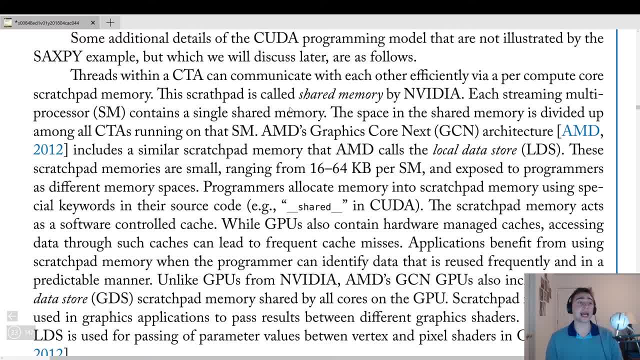 So GPUs have a very, very fast piece of memory we can access. that's local to the cores And it's called shared memory for NVIDIA GPUs And it's called the local data store for AMD GPUs in the GCN or graphics core, next architecture. 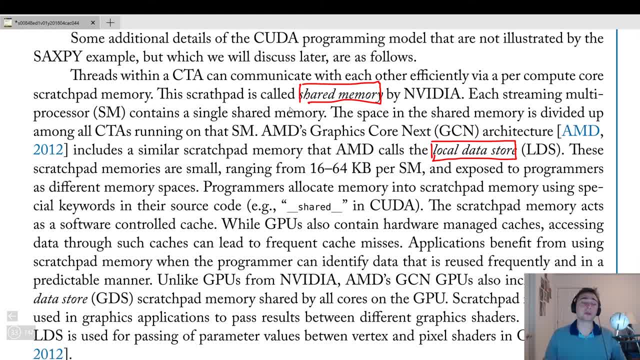 So what is shared memory? And you'll see this a lot if you start looking at optimized GPU code. So you should be familiar with something like a cache inside of a CPU, right? So GPUs have caches too, But the problem is because there's so many threads inside of a GPU. you have lots of threads all doing loads or stores. 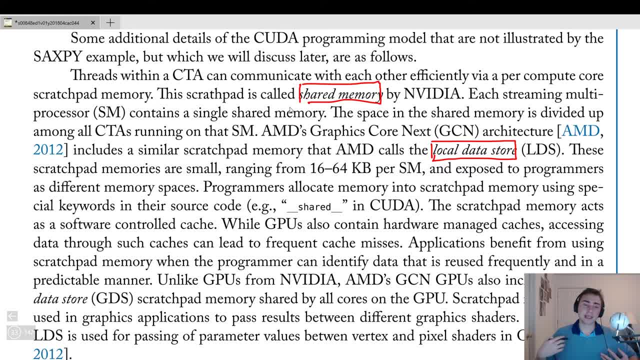 And you can have problems of locality. right, Because CPUs you have a single thread kind of going and it can find a good amount of locality. But as soon as you start putting more and more threads in you can have problems with locality. 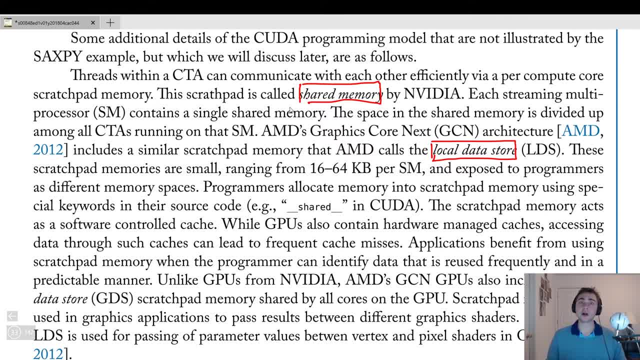 As soon as you start putting more threads active at the same time, they'll all be competing for the same cache And you can lose a lot of locality there. But what if you know exactly what kind of or what piece of data you needed to have locally at a given time? 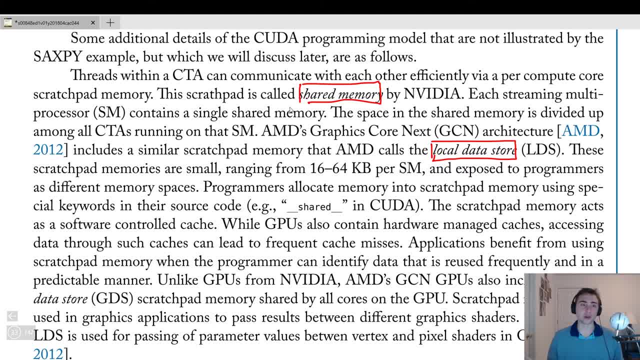 And you know you don't want those to get evicted, no matter what. So NVIDIA and AMD both allow this and something called shared memory or the local data store, which is the scratchpad memory, And what you can do with this is 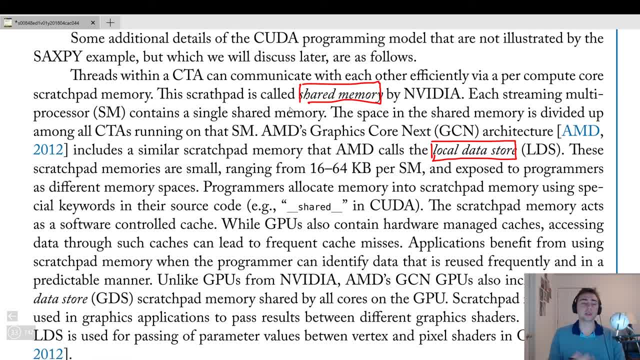 you can manually load data into scratchpad memory, which is very, very fast. It'll be like a five cycle access time, That is, you know you can access it in parallel with every thread of, like a warp, And you know it's not going to get evicted. 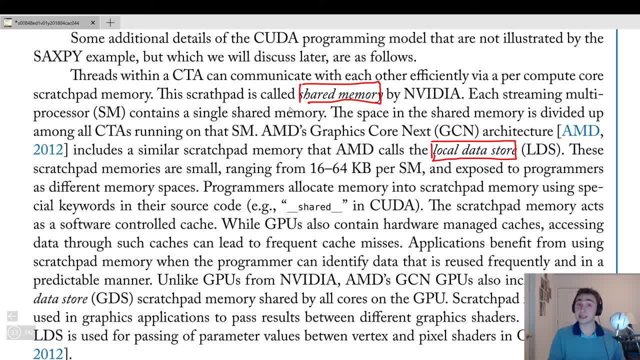 You manually, you know in the programming language itself. you know you have an interface to loading into the shared memory or local data store And also you know you can read and write from the local data store And you can also, you know, read from the local data store or scratchpad memory and write it back up to main memory. 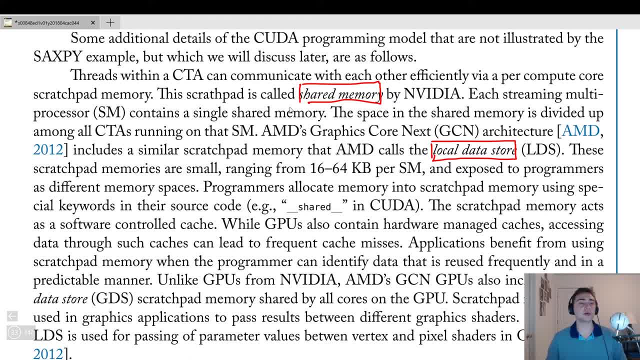 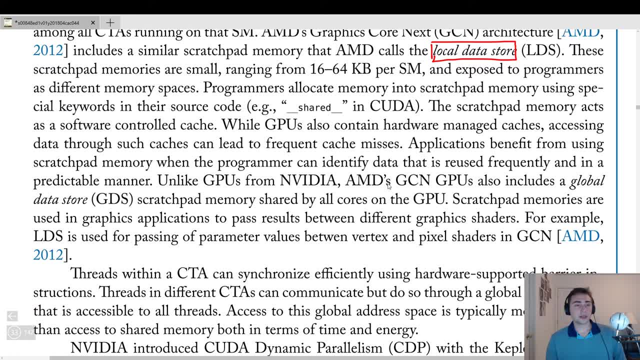 But it's kind of manually managed And so that's just kind of this optimization thing that we can do in a lot of GPU programs. So yeah, so this is typically for if the programmer can identify data that is reused frequently in a predictable manner. 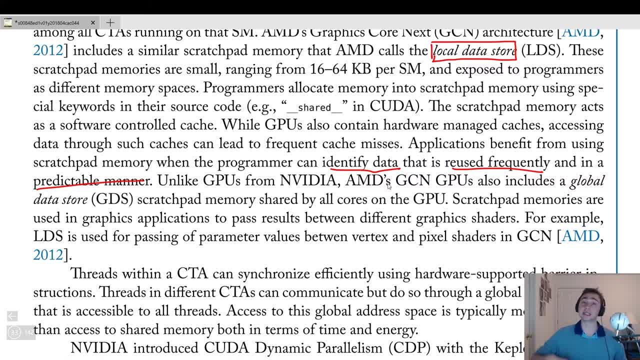 If it's not predictable, then you're not going to see much benefit because fundamentally you have to load from main memory, No matter what And before it goes into the local data store- scratchpad memory or shared memory- you know- it still requires you to load it from main memory. 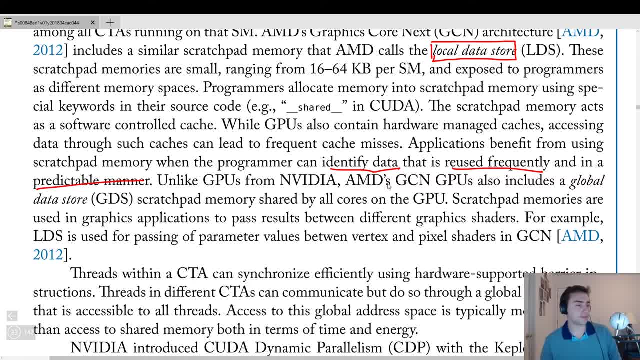 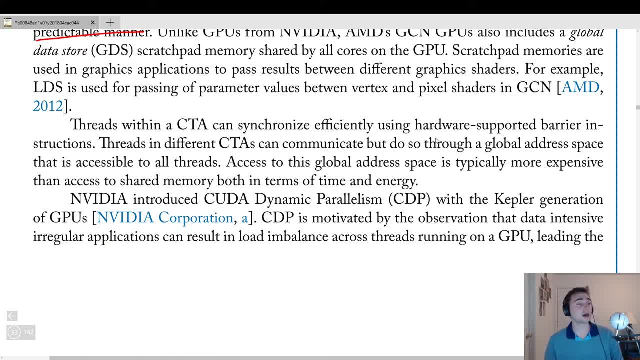 That's where the data is OK. So then you know, inside of a specific thread block- or CTA as they're often called- you can synchronize the threads within a single thread block. So there are supported barrier operations like underscore, underscore sync threads. 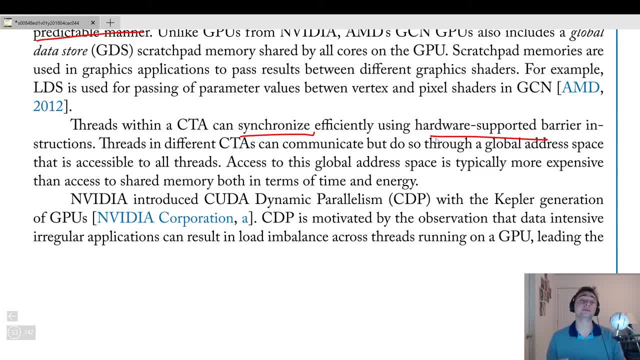 That says I will wait at this point, or every thread will wait at this point until every other thread of the thread block reaches here, And this is needed a lot of times when we're working with shared memory, Another interesting part of the programming language itself. 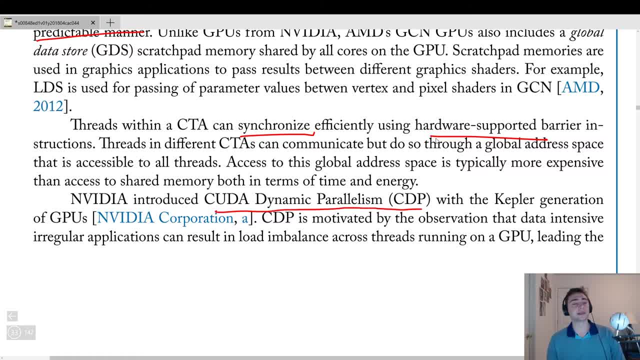 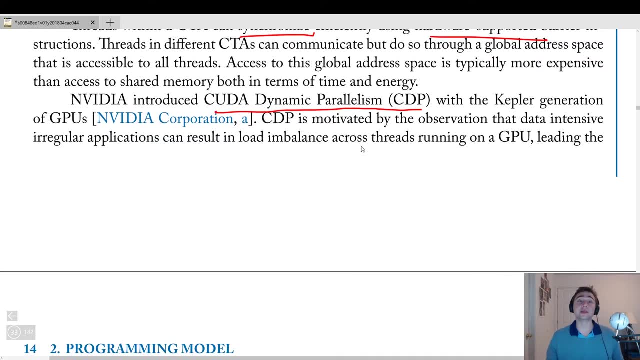 So NVIDIA introduced this thing called CUDA dynamic parallelism. So what is CUDA dynamic parallelism? So if we know, So we can. So CUDA dynamic parallelism just kind of enabled the ability to launch work on a GPU from the GPU, So no longer just has to come from the CPU launching work. 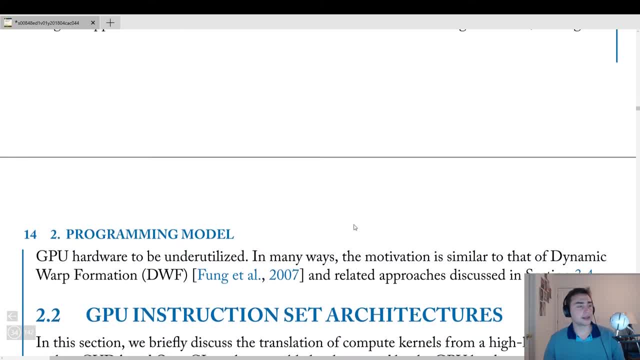 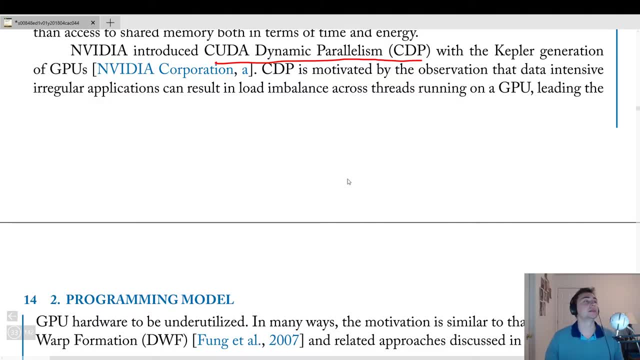 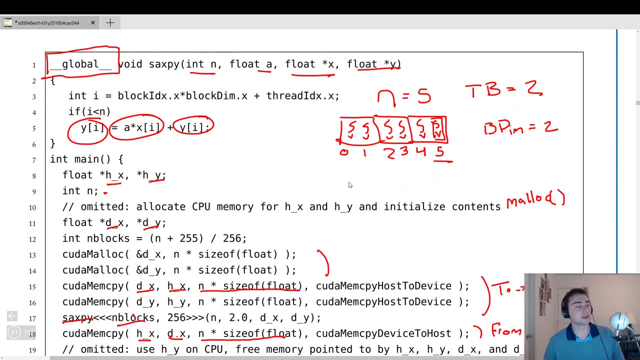 OK, So that's going to go ahead and do it for this episode. So that's kind of the fundamentals of GPU programming. So let's kind of wrap this up. So what we kind of saw was that, you know, fundamentally in a GPU application it starts with an allocation of memory, a copy of memory. 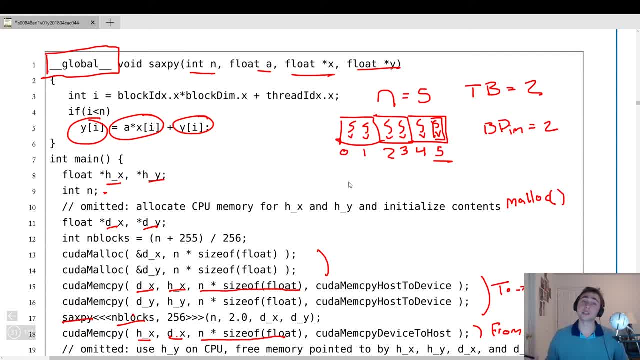 Then we have to define our problem right. So we map a problem- In this case it was Saxby- We map it to a grid of scalar threads, Think it's broken up into thread blocks. Then, with inside the kernel itself, every thread has to find where it is in this grid of thread blocks. 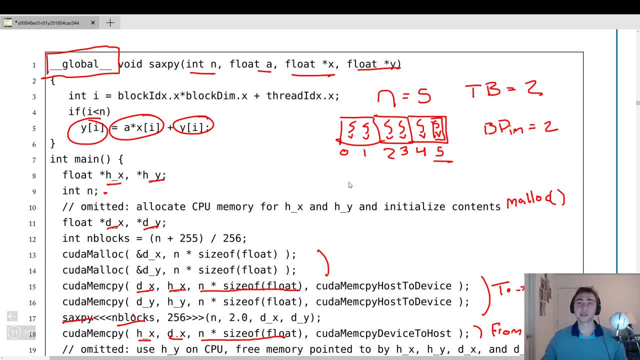 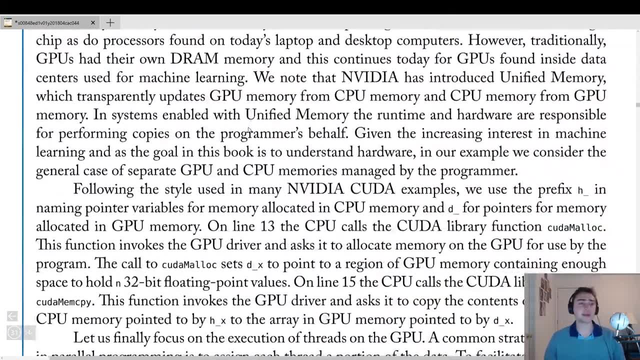 And then it will operate on the data that's mapped To that grid of thread blocks, Right, And that's that's managed by the programmer Theirself. And then we also talked a little bit about the fact we can have, You know, we can have- some slight optimization. 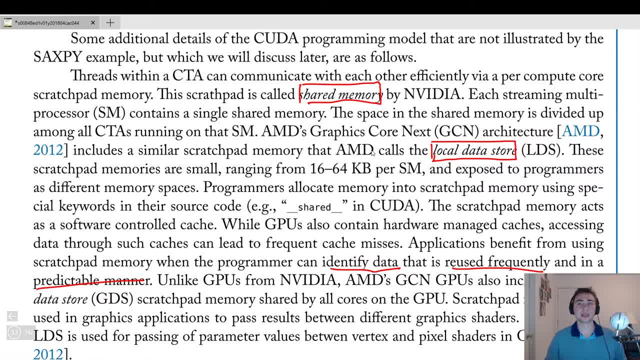 So if we want to exploit some, If we know exactly what data that we're going to be working on, we can of course have. We can of course have shared memory or local data score data store, frequently called scratchpad memory. 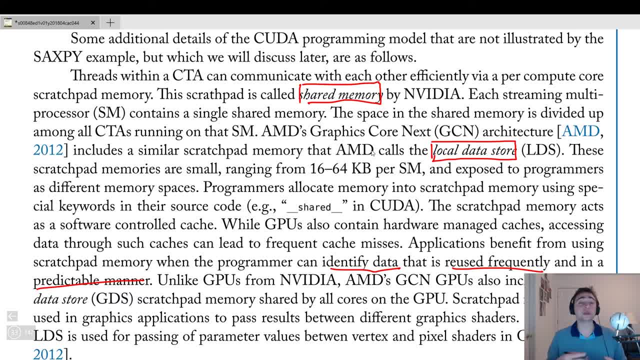 where we can put pieces of data That you know into a user managed L1 cache so that we can exploit locality that the programmer knows ahead of time. Right, And then we also talked a little bit about, you know, not only can we launch work from the CPU, 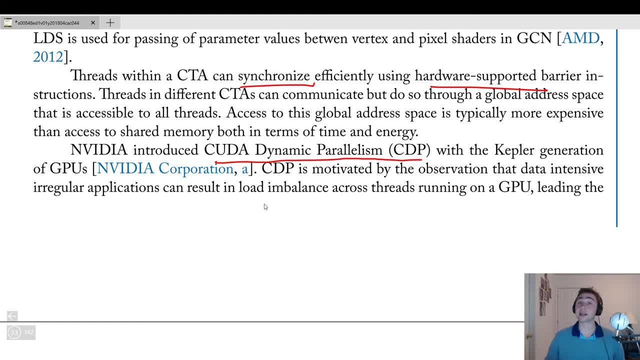 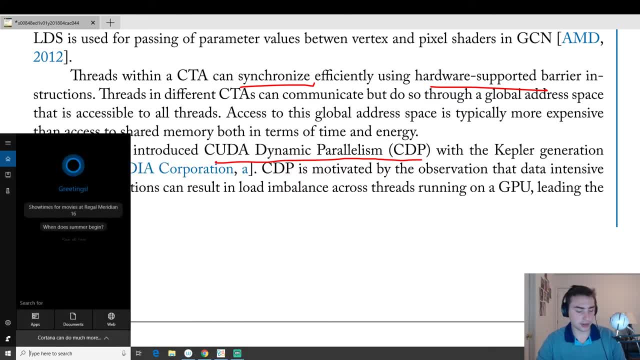 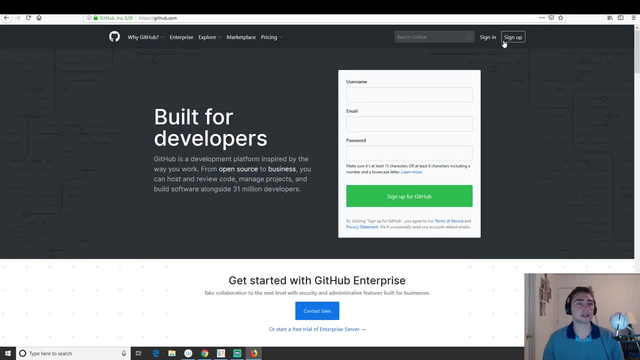 but with the introduction of CUDA, dynamic parallelism, we can actually launch work from the GPU itself. But OK, that's going to do it for this time, So let's go ahead and wrap it up. So feel free to go To go on the GitHub page at GitHub dot com. slash coffee before arch. 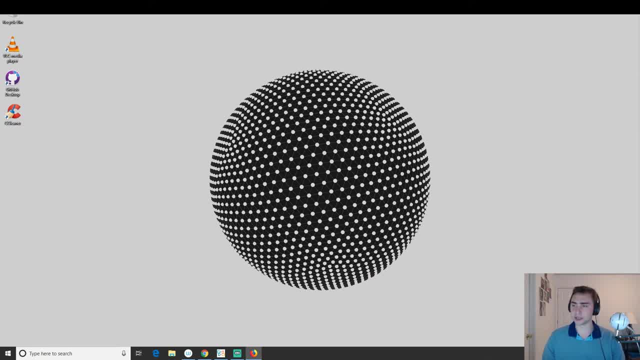 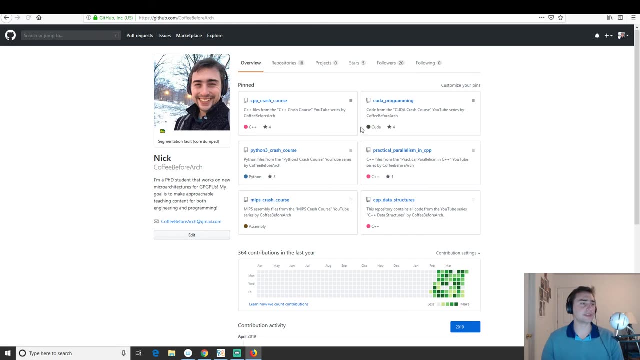 And I'm not logged in, So let me log in real quick. So on this page, this is where I do all of my, I host all of my code for all of my videos, And so feel free to download any of this. So I've got stuff on. you know, what's most related to this will be the CUDA programming stuff.